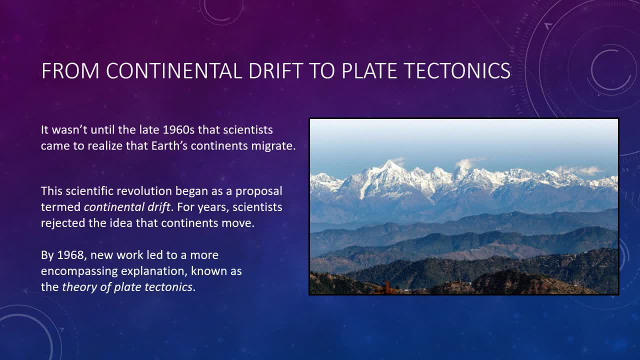 the seafloor, plunge deep into Earth's mantle. In short, a dramatically different model of Earth's tectonic processes emerged. Tectonic processes, where tecto means to build, are processes that deform Earth's crust to make major structural features such as mountains, continents and ocean basins. 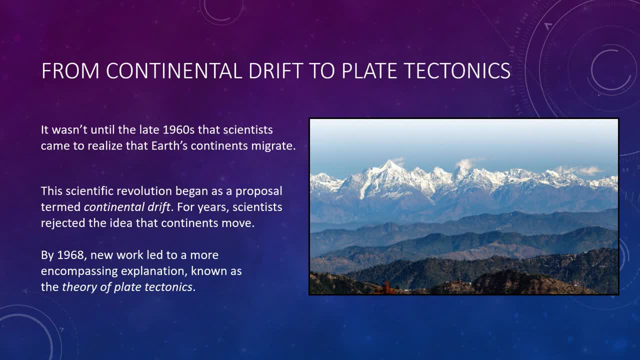 This profound reversal in scientific thought has been appropriately called a scientific revolution. The revolution began early in the 20th century as a relatively straightforward proposal termed continental drift. For more than 50 years, the scientific community categorically rejected this idea that continents are capable of movement. After World War II, modern instruments 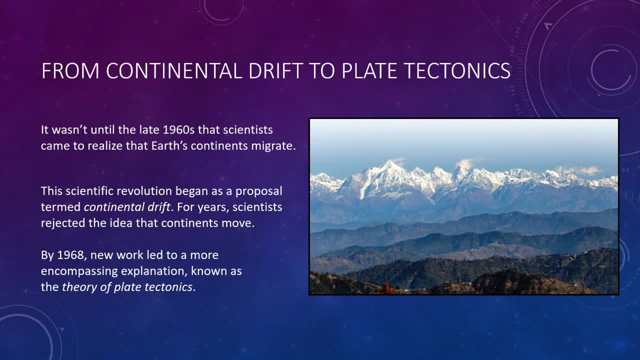 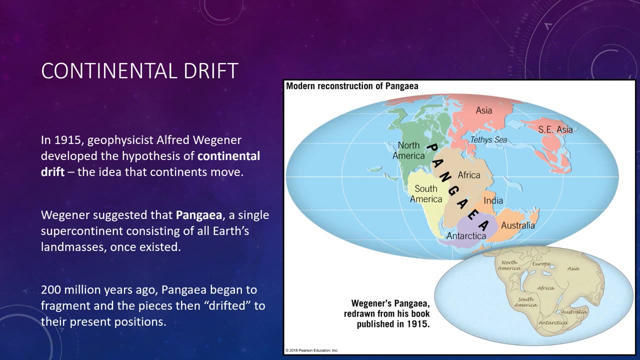 replaced rock hammers as tools of choice among many Earth scientists. By 1968, these developments had led to the unfolding of far more encompassing explanations, known as the theory of plate tectonics. During the 1600s, as better world maps became available, people noticed that continents 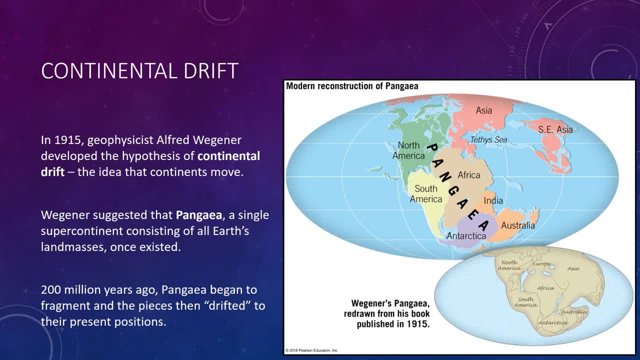 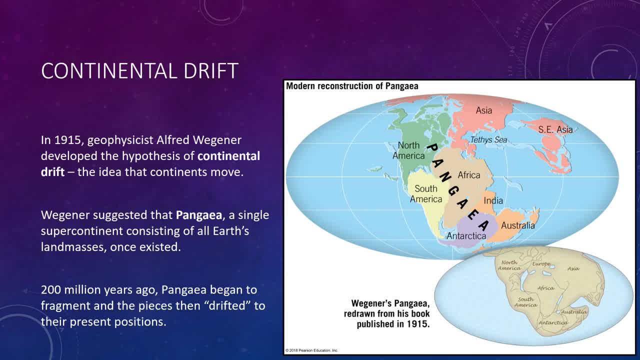 book outlined Wagner's hypothesis that continents and oceans were the origin of the ocean. This book also outlined a complete exponents' hypothesis called continental drift, which dared to challenge the long-held assumption that continents and ocean basins had fixed geographic positions underlying Geoscience. Waggoner suggested that a single supercontinent 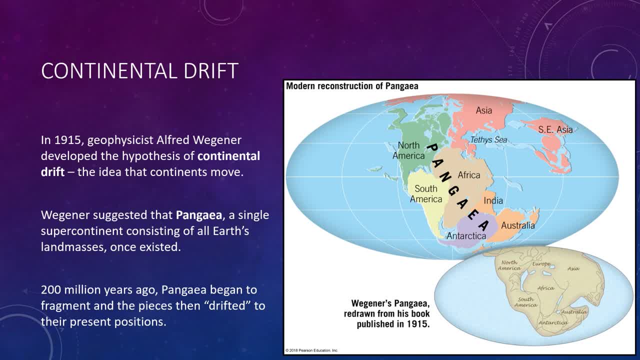 once existed. He named this giant landmass Pangea ice w preset geography as an breedingInstead of Earth's subspecies. 기억 on theあっ yolks vagy tahun. Allê, allê alê Amnestá EH. this supercontinent began to fragment into smaller landmasses. 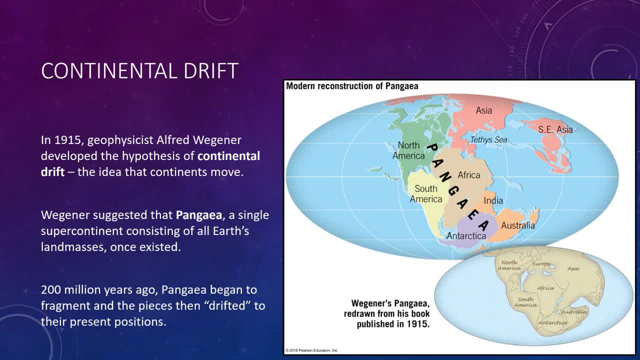 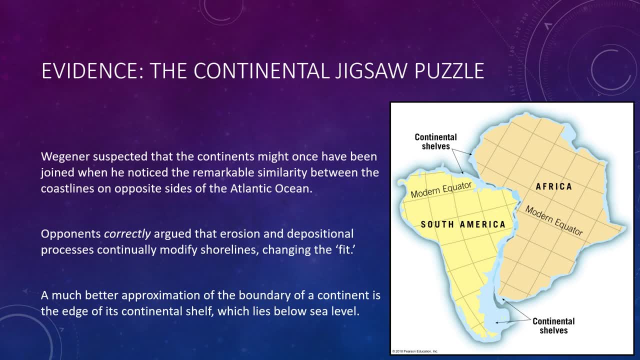 These continental blocks then drifted to their present position over a span of millions of years. So we're going to look at a few pieces of evidence for the continental drift idea. First, Wagner suspected that the continents might once have been joined when he noticed the remarkable similarity between the coastlines of the opposite sides of the Atlantic Ocean. 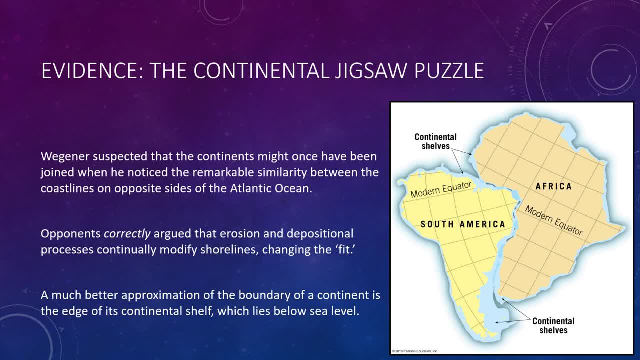 However, other Earth scientists challenged Wagner's use of present-day shorelines to fit these continents together. These opponents correctly argued that wave erosion and depositional processes continually modify our shorelines. Even if continental displacement had taken place, a good fit today would be unlikely. 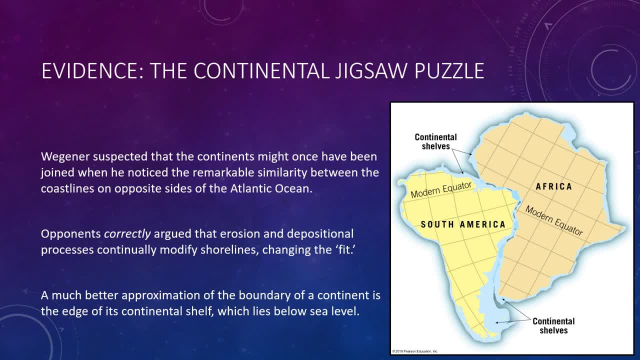 Scientists later determined that a much better approximation of the outer boundary of a continent is the seaward edge of its continental shelf, which lies submerged a few hundred meters below sea level. This is quite seriously like the drop-off in Finding Nemo. So this is the edge of the continental shelf that you see outlined in blue. 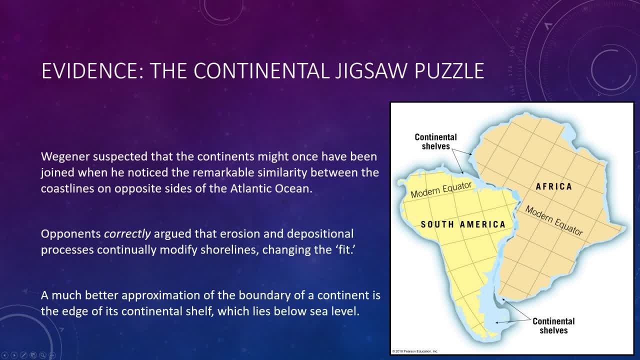 Those are what happen to fit together very well. In the early 1960s Sir Edward Bullard and two associates constructed a map that pieced together the edges of the continental shelves of the continents of South America and Africa at a depth of about 3,000 feet. 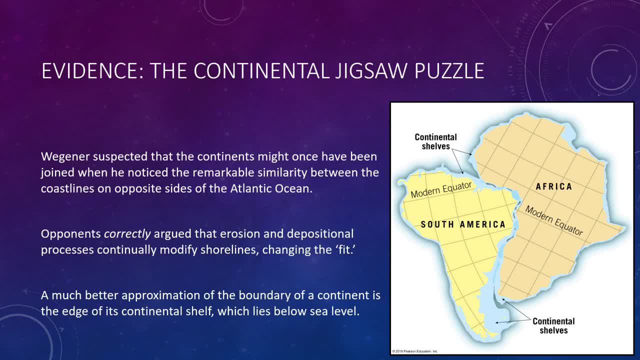 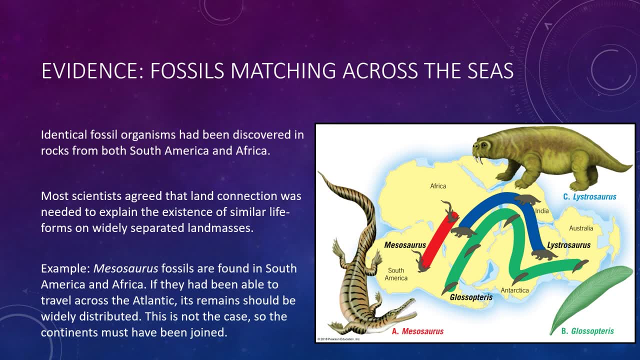 The remarkable fit obtained was more precise than even researchers had expected. It was when Wagner learned that identical fossil organisms had been discovered in rocks from both South America and Africa that his pursuit of continental drift became more focused. Wagner learned that most paleontologists agreed. 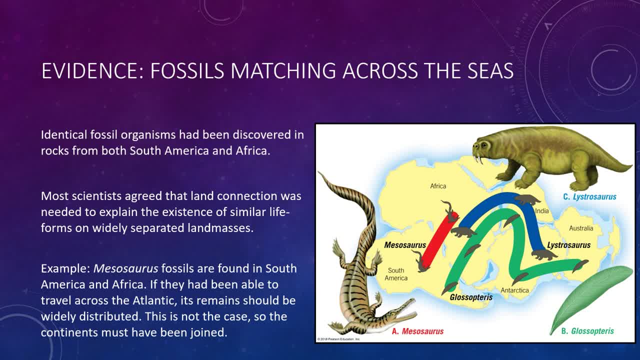 that some type of land connection was needed to explain the existence of similar Paleozoic Age lifeforms on widely separated landmasses. Just as modern lifeforms native to North America are not the same as those in Africa and Australia Paleozoic Age organisms on widely separated continents. 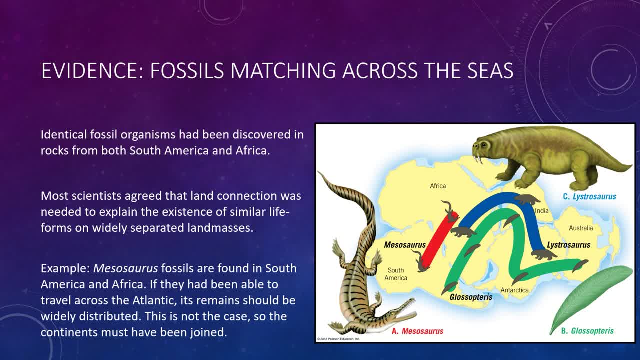 should have been distinctly different. Wagner documented several cases in which the same fossil organism is found on landmasses that are now widely separated, even though it is unlikely that the living organism could have crossed the barrier of a broad ocean. A classic example is the Mesosaurus. 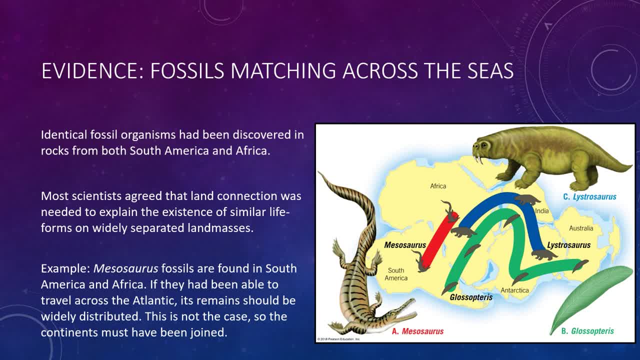 a small aquatic freshwater reptile whose fossil remains are mainly found in shales of Permian Age rocks in eastern South America and in the Pacific Ocean, in eastern South America and in the Pacific Ocean, in eastern South Africa and in the Pacific Ocean. 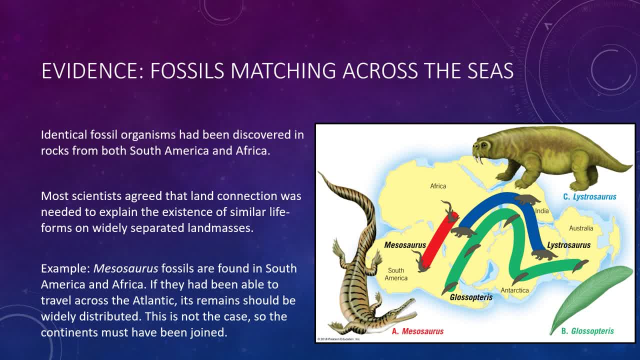 If Mesosaurus had been able to make the journey across the South Atlantic, its remains should be more widely distributed. Because this is not the case, however, Wagner asserted that South America and Africa must have been joined together during that period of history. 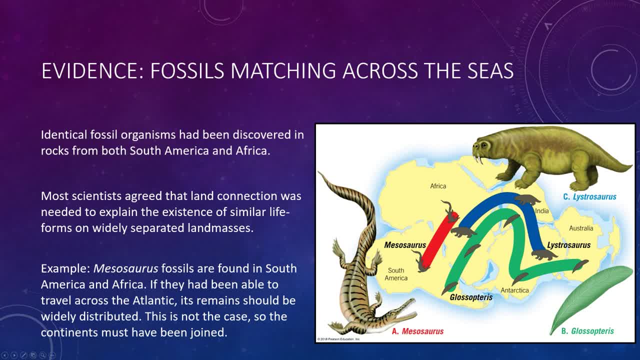 So this animal, the Mesosaurus, was not able to cross an entire ocean, and even if it did, we would see its fossils all over the place. Well, we don't. We only saw it in a very thin region connecting South America and Africa. 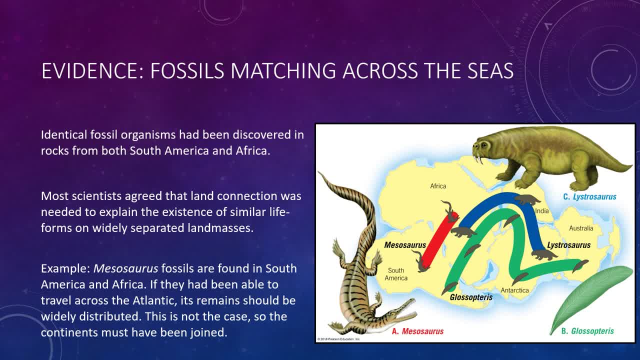 Wagner also cited the distribution of the fossil seed ferns Glossopterus as evidence for Pangea's existence. So you can see that in the bottom right, With tongue-shaped leaves and seeds too large to be carried by wind. 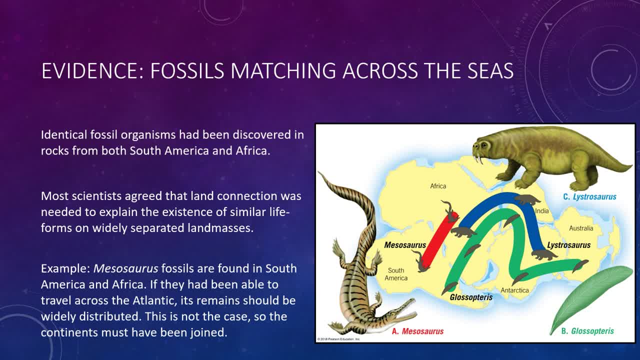 this plant was known to be widely dispersed throughout Africa, Australia, India and South America. Later, fossil remains of Glossopterus are also discovered in Antarctica. Wagner also learned that the seed, ferns and associated flora grew only in cold climates. 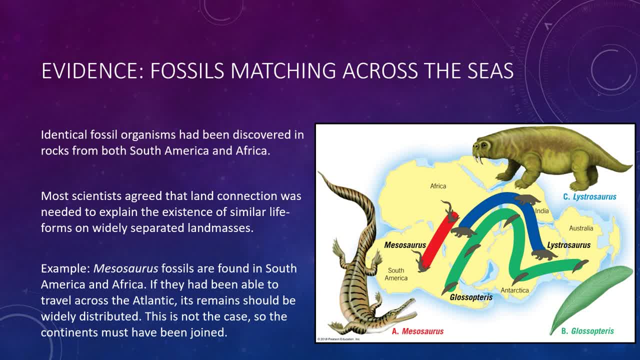 similar to central Canada. Well, therefore, he concluded that when these landmasses were joined, they were located much closer to the South Pole. So again, this is an example that, if we have the present-day structure of our continents, this leaf is too heavy. 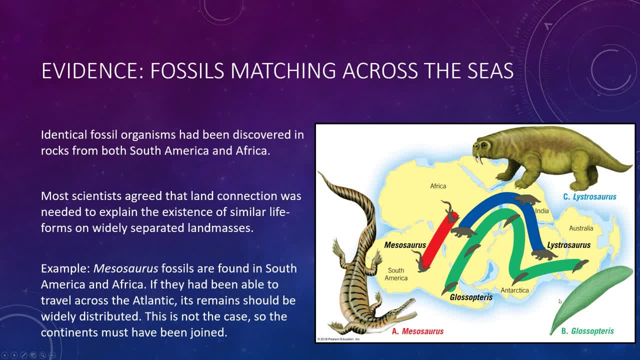 or shaped too poorly for it to travel across an entire ocean. So the fact that we find its fossil remains all across different continents is indicative of the fact that they were once connected. Furthermore, they only grow in cold climates. Well, Central Africa is not very cold today. 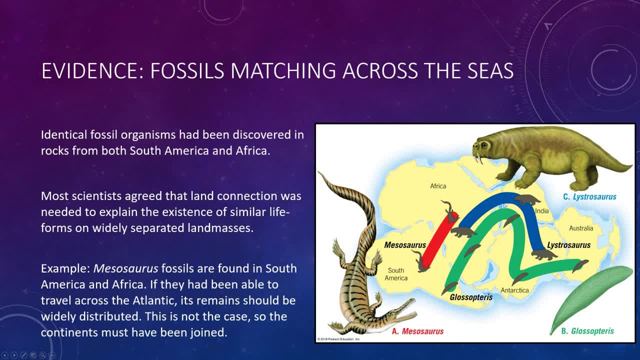 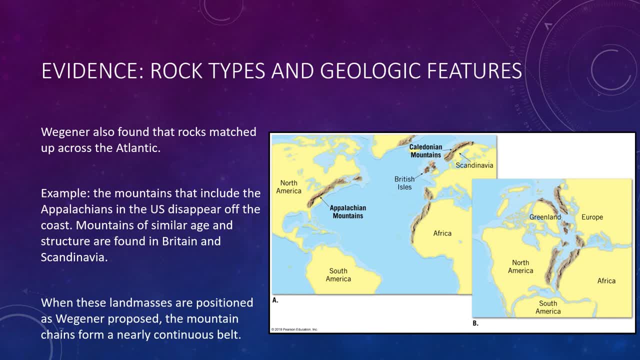 Australia not very cold today. So it's believed that not only were they connected, but connected close to the South Pole, where it was colder in the past. Wagner also found that rocks matched up across the Atlantic Ocean, For instance highly deformed igneous rocks in Brazil. 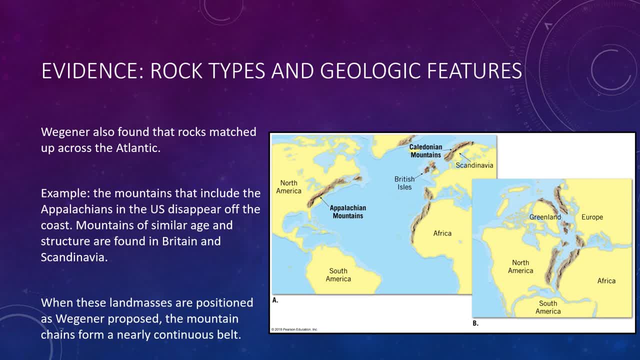 closely related to the South Pole, closely resemble similar rocks of the same age in Africa. Also, the mountain belt that includes the Appalachians tends toward the northeast through the eastern United States and disappears off the coast of Newfoundland- Mountains of comparable age and structure. 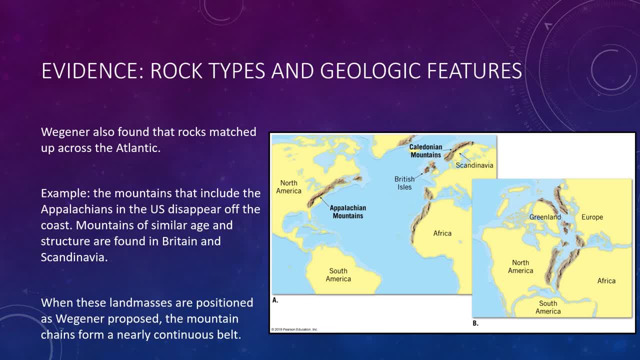 are found in the British Isles in Scandinavia. When these landmasses are positioned as Wagner proposed, the mountains form a chain of nearly continuous belt, as you can see in image B. As Wagner wrote, quote: it is just as if we were to refit the torn pieces of a newspaper. 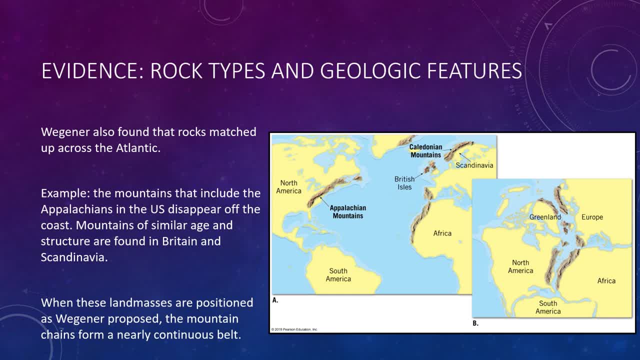 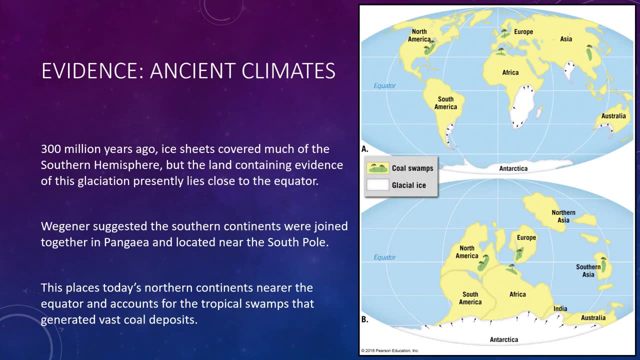 by matching their edges and then to check whether the lines of print run smoothly across. If they do, there is nothing left but to conclude that the pieces were in fact joined this way About 300 million years ago. vast ice sheets covered extensive portions. 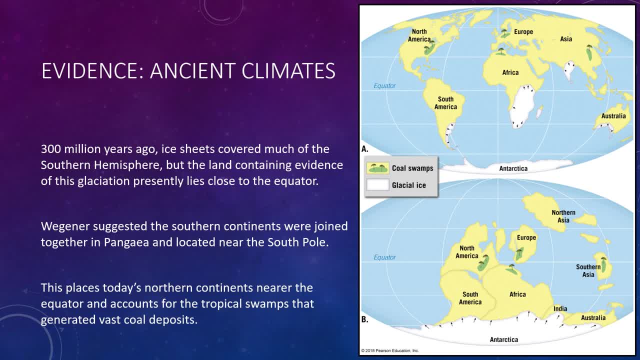 of the southern hemisphere, as well as India. Much of the land area that contains evidence of this paleozoic glaciation presently lies within 30 degrees of the equator, in subtropical or even tropical climates. So how could extensive ice sheets form near the equator? 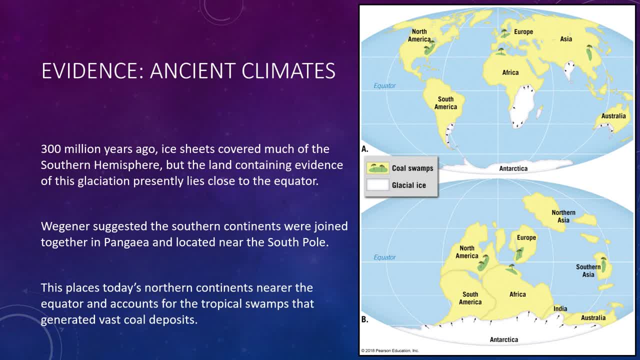 One proposal suggested that our planet experienced a period of extreme global cooling. Wagner rejected this explanation because during the same span of geological time, large tropical swamps existed in several locations in the northern hemisphere. The lush vegetation in those swamps was eventually buried and converted to coal. 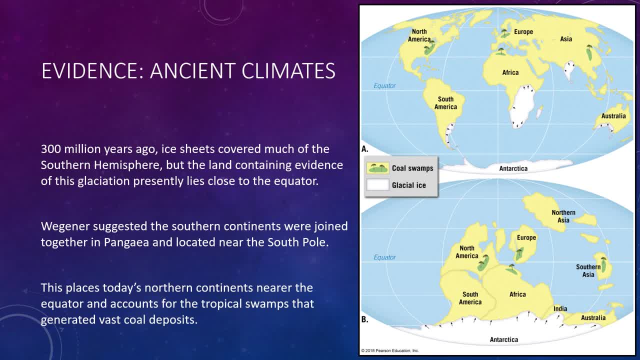 Today, these deposits comprise major coal fields in the eastern United States and northern Europe. Many of the fossils found in these coal-bearing rocks were produced by tree ferns with large fawns, ferns that would have grown in warm, moist climates. The existence of these large tropical swamps 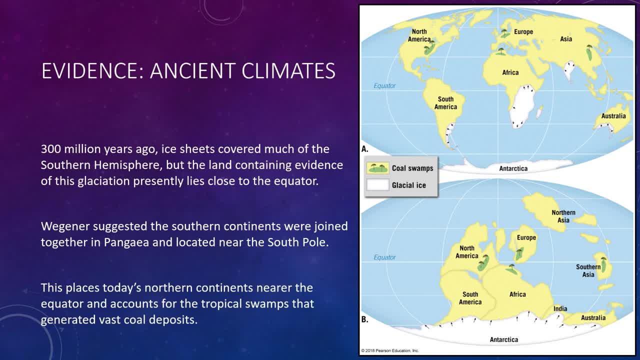 Wagner argued was inconsistent with the proportionality, and he proposed that extreme global cooling caused the glaciers to form in areas that are currently tropical. Wagner suggested a more plausible explanation for the late paleozoic glaciation, As we mentioned in the previous slide. 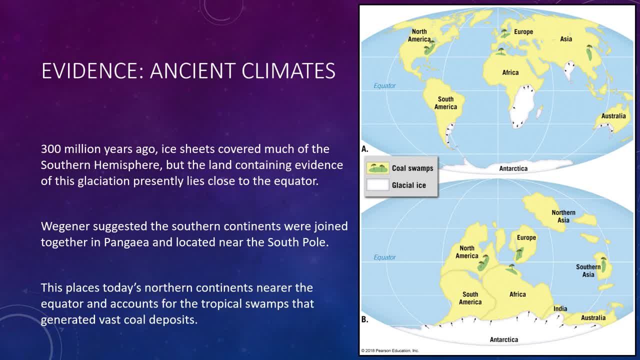 the southern continents were joined together in the supercontinent of Pangaea and located near the South Pole. This would account for the polar conditions required to generate extensive expanses of glacial ice over much of these landmasses. At the same time, this geography places today's northern continents 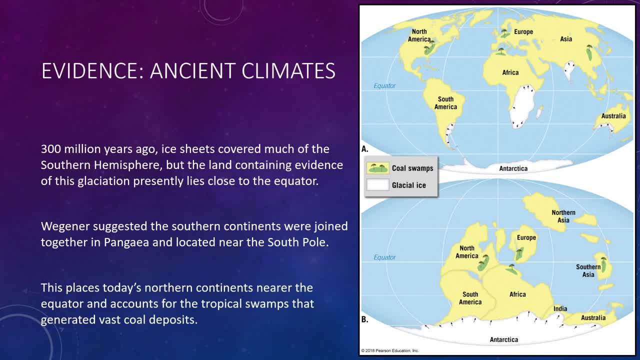 nearer the equator and accounts for the tropical swamps that generated vast coal deposits. So if you look at this image, a lot of this glacial evidence occurs near the equator. I mean Central Africa is very warm. Australia and India both get very warm in these equatorial regions. 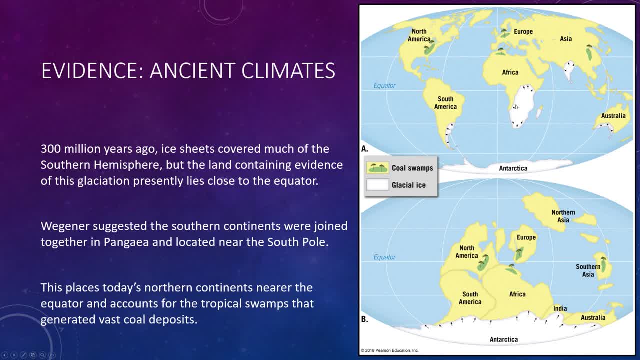 So they couldn't have always stayed this way, because glaciers wouldn't exist over half of Africa today. So he proposed that all of those glaciers or filled regions were connected further down near Antarctica, as you see here. This also would explain the nature of our coal beds that we find. 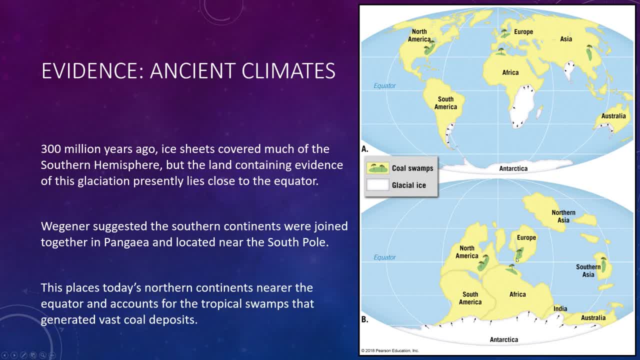 This placed parts of North America and Europe along the equator, where it was warm and moist, and so tropical regions formed a lot of swamps. Then those swamps decayed and left behind their remnants, and then the continents moved to their current positions. 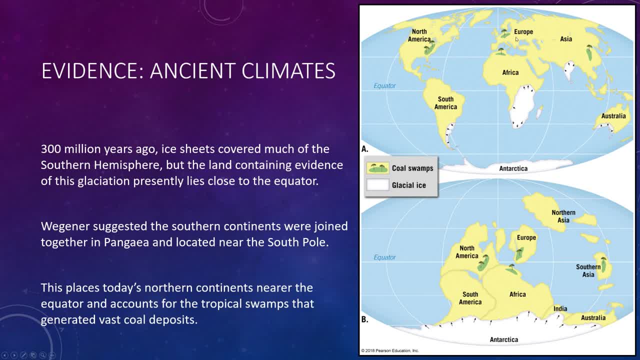 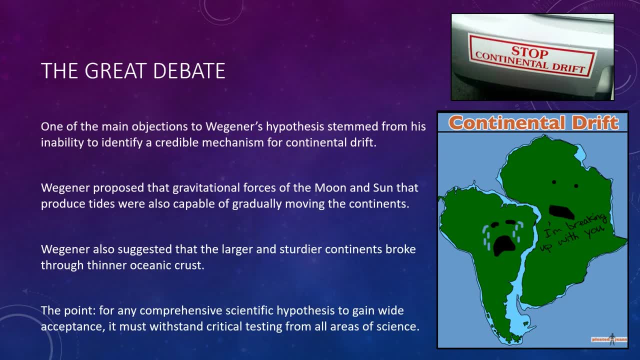 and now we see the coal beds in place in parts of North America and around the Mediterranean. From 1924, when Wagner's book was translated into English, French, Spanish and Russian, until his death in 1930,, his proposed drift hypothesis encountered a great deal of hostile criticism. 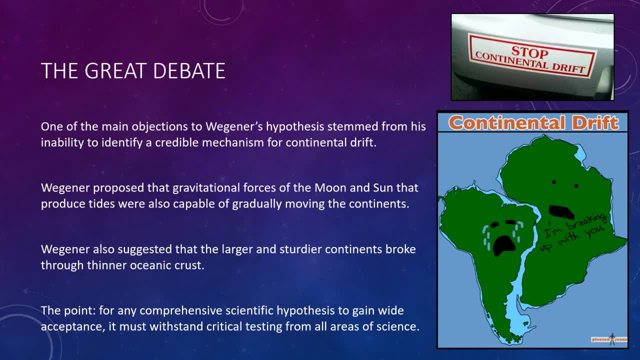 One of the main objections to Wagner's hypothesis stemmed from his inability to identify a credible mechanism for continental drift. Wagner proposed that gravitational forces of the moon and sun that produced the energy of the sun that produced Earth's tides, were also capable of producing moving continents across the globe. 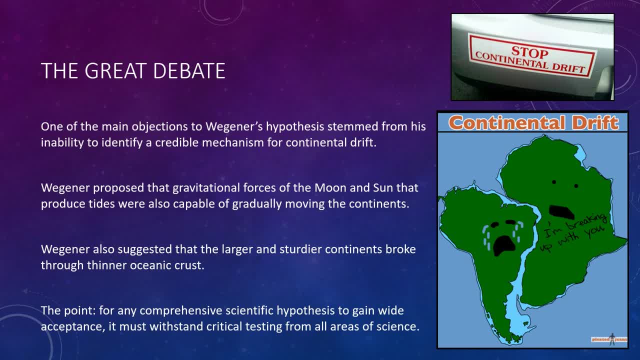 However, the prominent physicist Harold Jeffries correctly argued that tidal forces strong enough to move Earth's continents would have resulted in halting our planet's rotation, which, of course, is not happening. Wagner also incorrectly suggested that the larger and sturdier continents broke through thinner oceanic crusts. 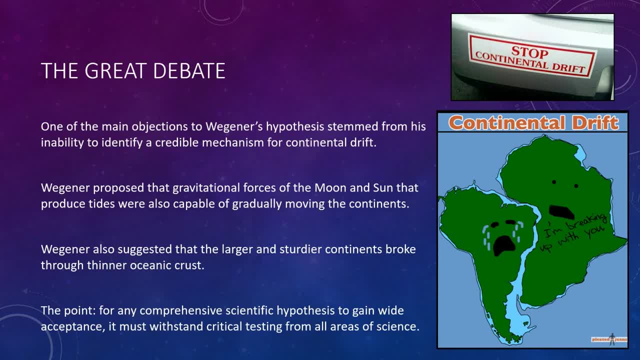 much like an icebreaker's ship breaks through ice. However, no evidence existed to suggest that the ocean floor was weak enough to permit passage of the continents without the continents themselves becoming appreciably deformed in the process, Why Wagner was unable to overturn. 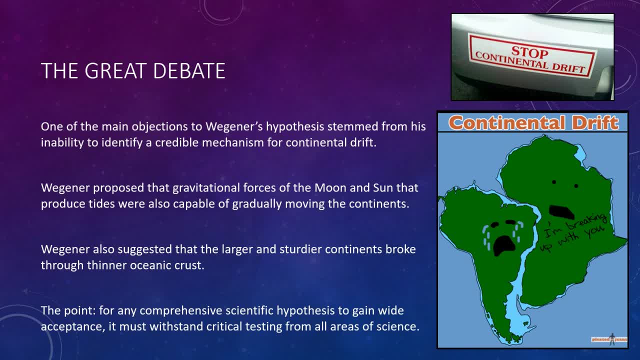 the established scientific views of his day is pretty straightforward. Foremost was the fact that, although the central theme of his drift hypothesis was correct, many details were not. So, for example, continents definitely do not break through the ocean floor, and tidal energy very much does not. 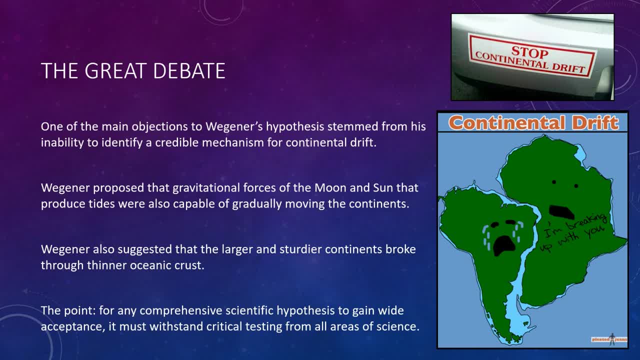 have enough strength to move the continents. Moreover, for any comprehensive scientific hypothesis to gain wide acceptance, it must withstand critical testing from all areas of science. Despite Wagner's great contribution to our understanding of Earth, not all of the evidence supported the continental drift hypothesis. 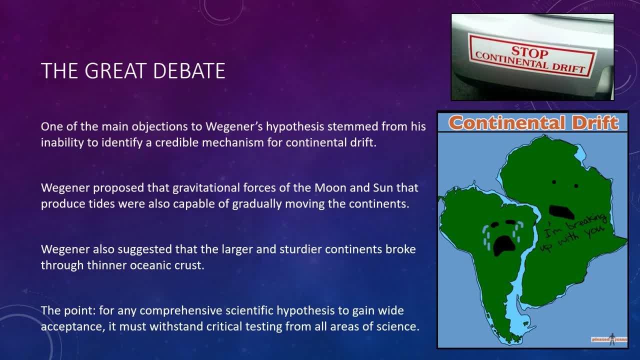 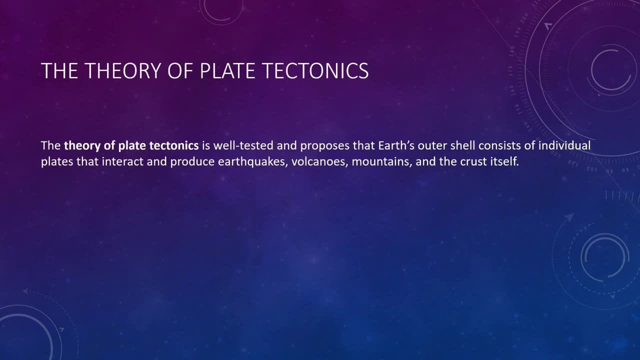 as he proposed it. As a result, most of the scientific community, particularly North America, rejected continental drift or at least treated it with considerable skepticism Following World War II. oceanographers equipped with new marine tools and ample funding from the US Office of Naval Research. 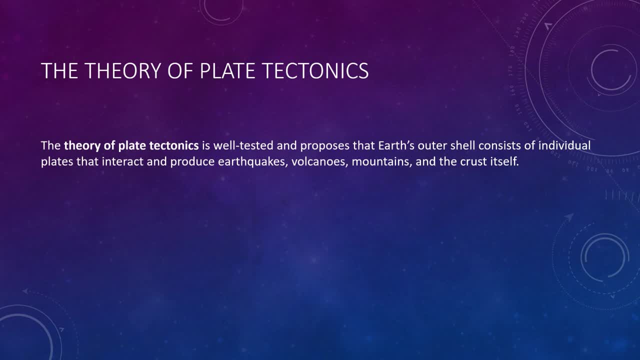 embarked on an unprecedented period of oceanographic research. Over the next two decades, a much better picture of large expanses of the seafloor slowly and painstakingly began to become emerged. From this work came the discovery of a global oceanic ridge system. 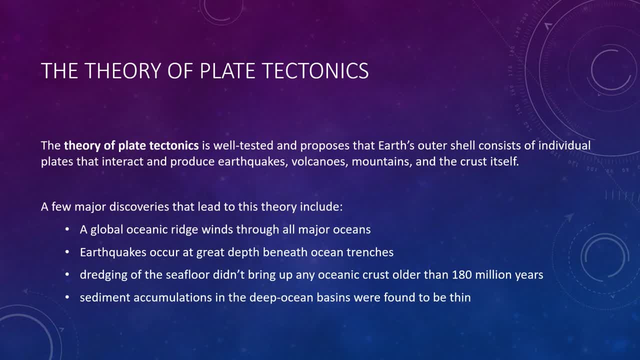 that winds through all the major oceans. So studies conducted in the western Pacific demonstrated that earthquakes were occurring at great depths beneath ocean trenches. Of equal importance was the fact that dredging of the seafloor did not bring up ocean crusts. that was older than the ocean. 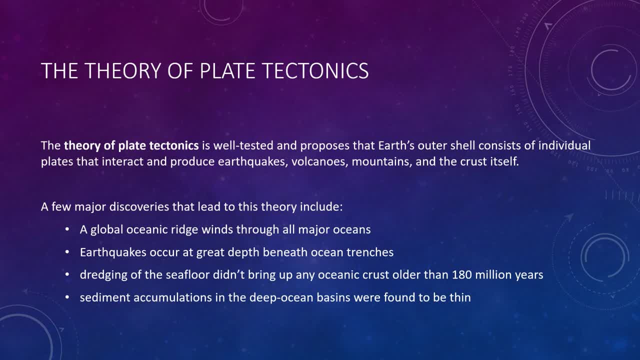 Dredging of the seafloor was a major part of the reason why the ocean was so large. The seafloor was larger than 180 million years old. More on that soon. Further sediment accumulations in the deep ocean basins. 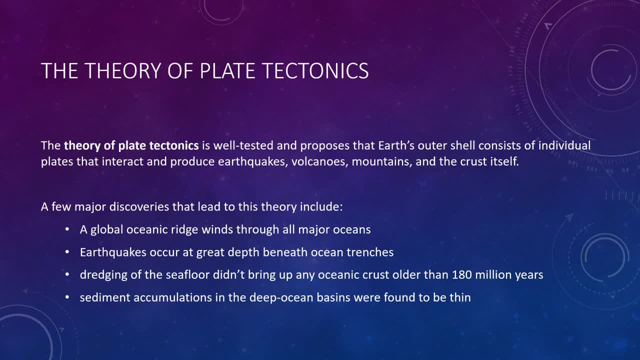 were found to be thin, not the thousands of meters that had been predicted By 1968,. these developments, among others, had led to the unfolding of a far more encompassing theory than continental drift, known as the theory of plate tectonics. 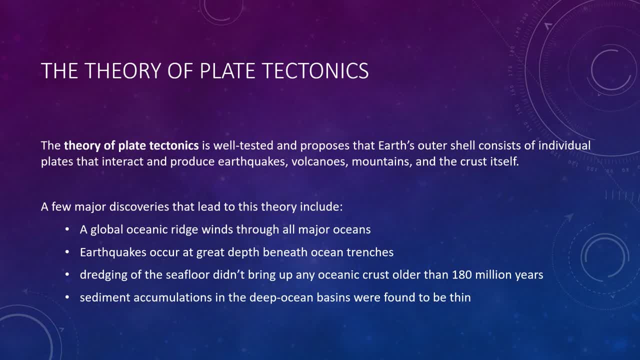 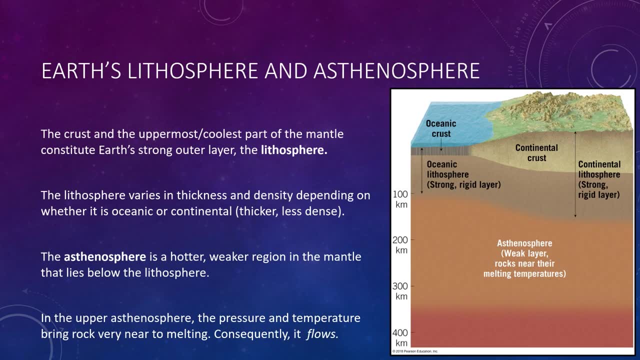 The theory of plate tectonics was the basis for the development of continental drift. The theory of plate tectonics was the basis for the development of continental drift. The theory of plate tectonics was the basis for the development of continental drift. 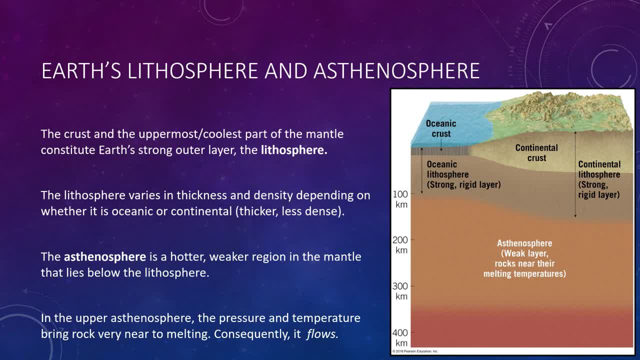 According to the plate tectonics model, the crust and uppermost, and therefore coolest, part of the mantle constitute Earth's strongest outer layer, the lithosphere. lithos standing for stone. The lithosphere varies in both thickness and density depending on 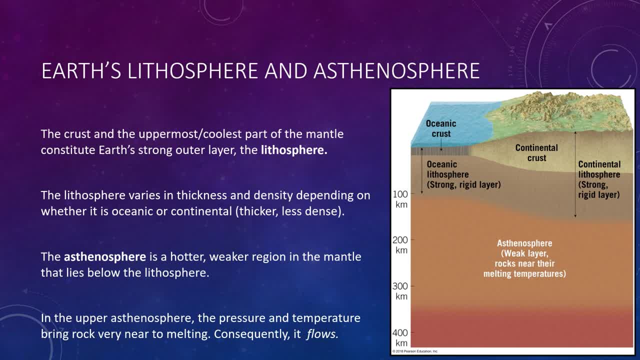 whether it is oceanic or continental. Oceanic lithosphere is about 60 miles thick in the deep ocean basins, but is considered to be the largest lithosphere in the world, According to the oceanic ridge system. the crust is considerably thinner along. 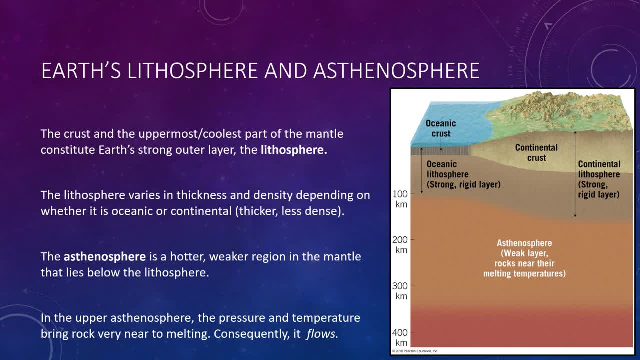 the crust of the oceanic ridge system. In contrast, however, continental lithosphere averages about 90 miles thick and may extend up to 125 miles or more beneath the stable interiors of the continents. Further, oceanic and continental crust differ in density. 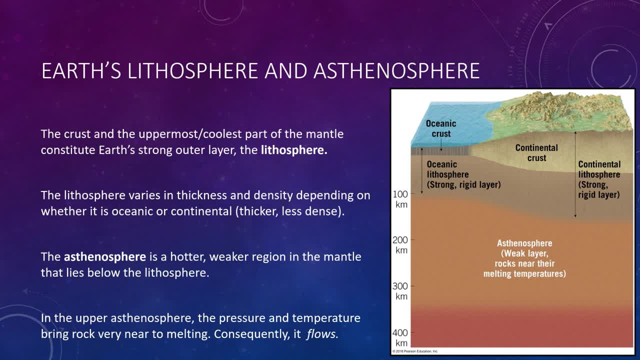 Oceanic crust is composed of basalt, whereas continental crust is composed largely of less dense granitic rock. Because of these differences, the overall density of oceanic lithosphere, that is, the crust and upper mantle, is greater than the overall density of the continental. 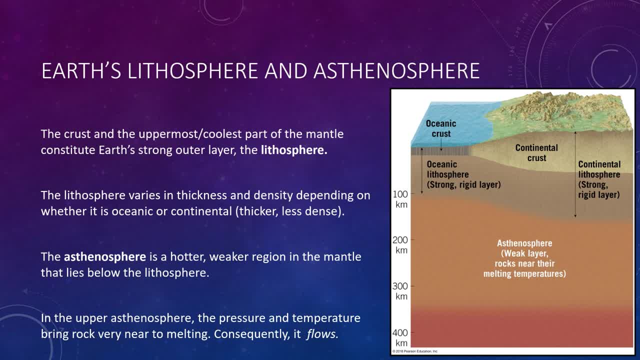 lithosphere. The athenosphere where athenos stands for weak, is a hotter and weaker region in the mantle that lies just below the lithosphere, In the upper athenosphere, which is located between 60 and 125 miles of depth. 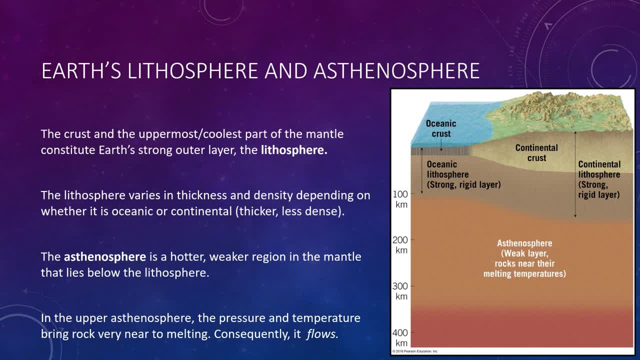 the pressure and temperature bring rock to a very near melting point. Consequently, although the rock remains largely solid, it responds to forces by flowing, similar to the way that clay may deform if you compress it slowly. By contrast, the relatively cool and rigid lithosphere 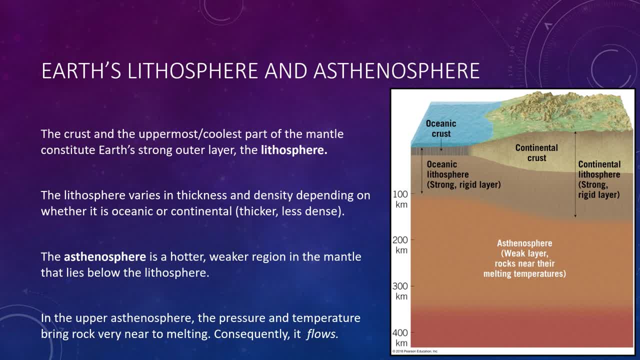 tends to respond to forces that act on it by bending or breaking so that it can move independently. Because of these differences, Earth's rigid outer shell effectively is detached from the athenosphere, which allows these layers to move independently. The lithosphere is broken. 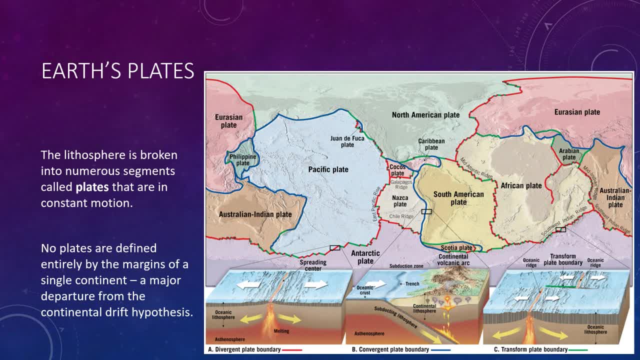 into numerous segments of irregular size and shape, called plates, that are located in constant motion with respect to one another. Seven major lithospheric plates are recognized and account for 94% of Earth's surface area: the North American, South American, Pacific, African. 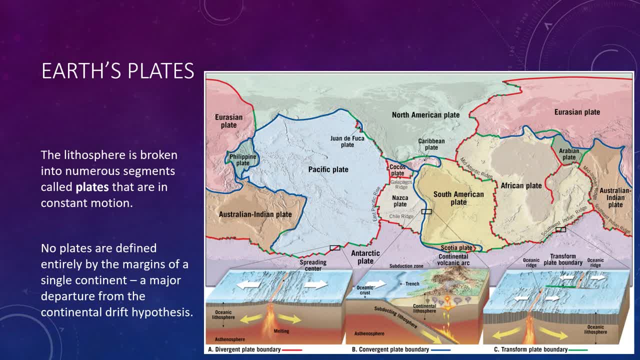 Eurasian, Australian-Indian and Antarctic plates. The largest is the Pacific plate, which encompasses a significant portion of the Pacific Basin. Each of the six other large plates consists of an entire continent, as well as a significant part of the South Atlantic. 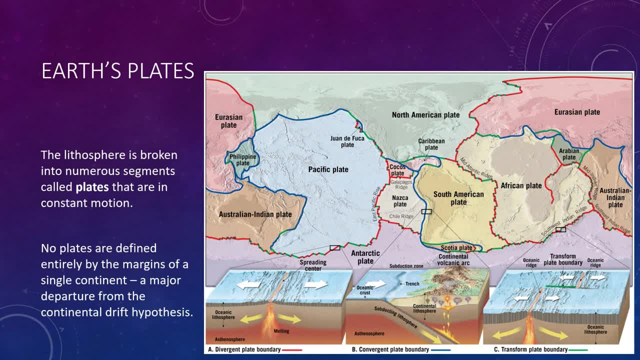 Notice that the South American plate encompasses all of South America and about one half of the floor of the South Atlantic. Note also that none of the plates are defined entirely by the margins of just a single continent. This is a major departure from Wagner's continental 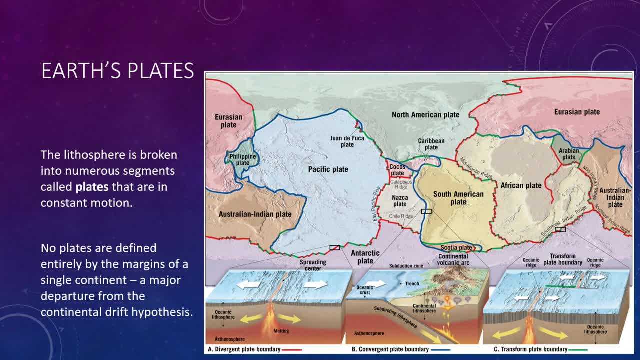 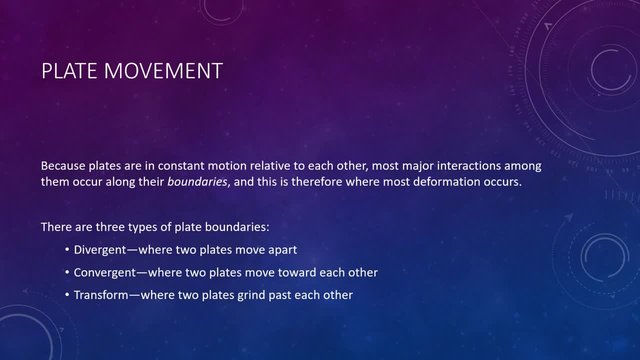 drift hypothesis, which proposed that continents move through the ocean floor, not with it. As plates move, the distance between two locations on different plates, such as New York and London, gradually changes, whereas the distance between two sites on the same plate. 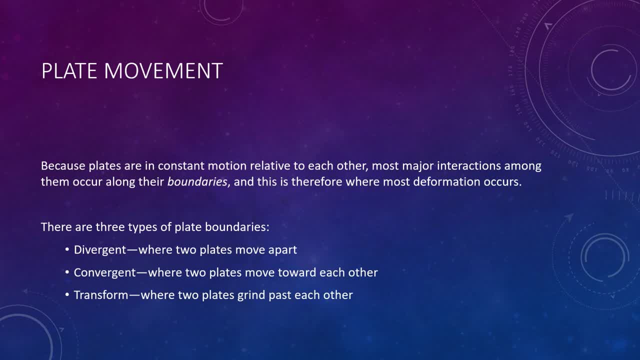 such as New York and Denver, for example, remain relatively constant. Because plates are in constant motion with one another, most major interactions among them occur along their boundaries, and this is therefore where most deformation occurs. Plates were first established by plotting the locations of 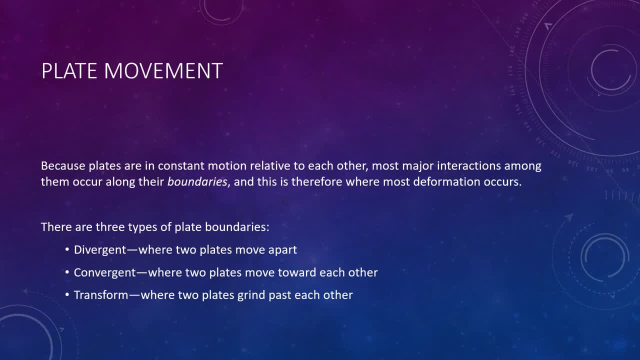 earthquakes and volcanoes. Plates are delimited by three distinct types of boundaries, which are differentiated by the types of movement they exhibit. The three types of plate boundaries, which we will look at in a lot more detail after this, are divergent plate boundaries. 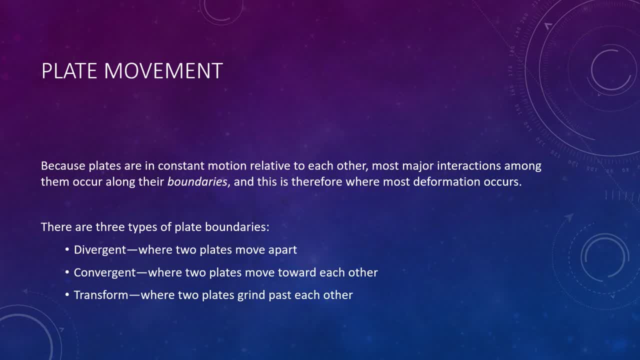 where two plates move apart, resulting in upwelling and convergent plate boundaries. where two plates move toward one another, resulting either in oceanic lithosphere descending beneath an overriding plate, eventually to be reabsorbed into the mantle, or possibly. 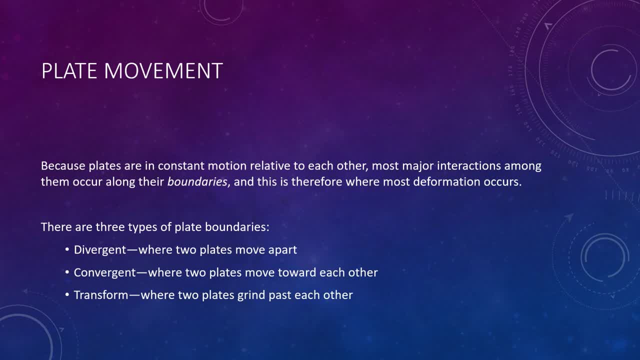 in the collision of two continental land masses to create a mountain belt. The third type is a transform plate boundary, where two plates grind past each other without the production or destruction of lithosphere. Divergent and convergent plate boundaries each account for about. 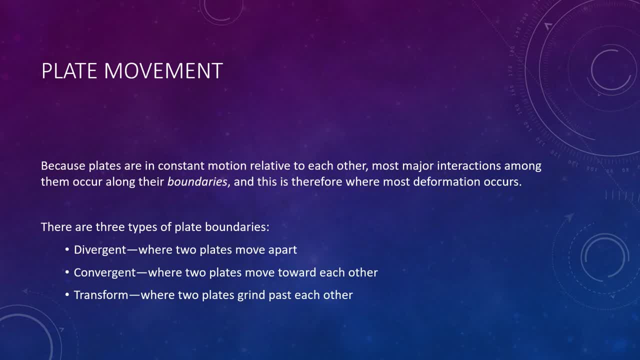 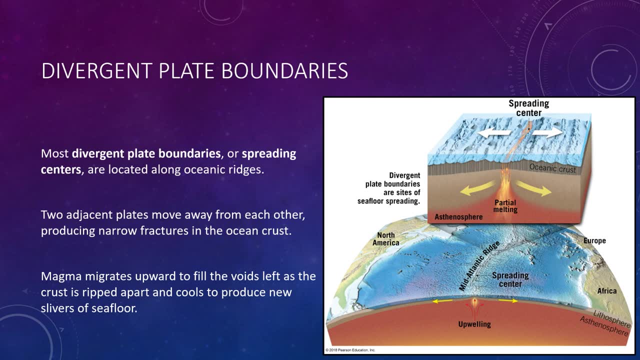 40% of all boundaries on Earth. Transform boundaries account for the remaining 20%. So let's first take a look at divergent plate boundaries for several slides. Most divergent plate boundaries, where di means apart and verge means to move, so to. 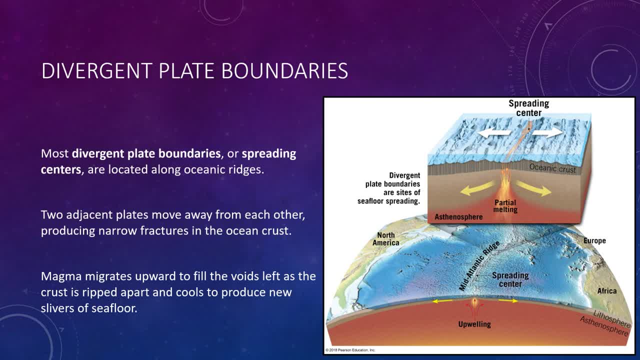 move apart are located along the crest of oceanic ridges and can be thought of as a constructive plate margin, because this is where new ocean floor is generated. Here, two adjacent plates move away from one another, producing a long, narrow fracture. 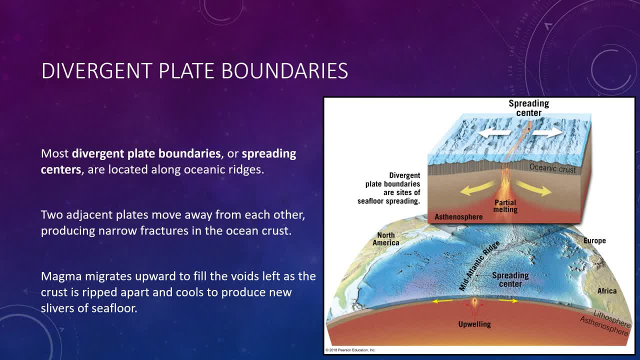 in the ocean crust. As a result, hot molten rock from the mantle below migrates upward to fill the void left as the crust is being ripped apart. This molten material gradually cools to produce new slivers of seafloor. 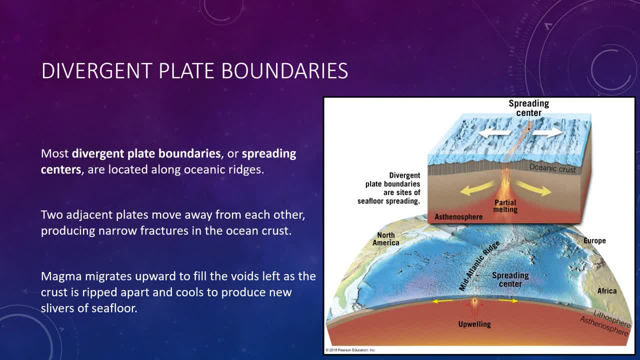 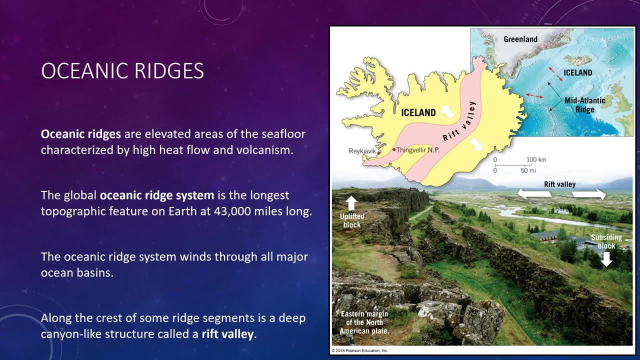 In a slow yet unending manner, adjacent plates spread apart. As a result, new oceanic lithosphere forms between them. For this reason, divergent plate boundaries are also called spreading centers. The majority of, but not all, divergent plate. 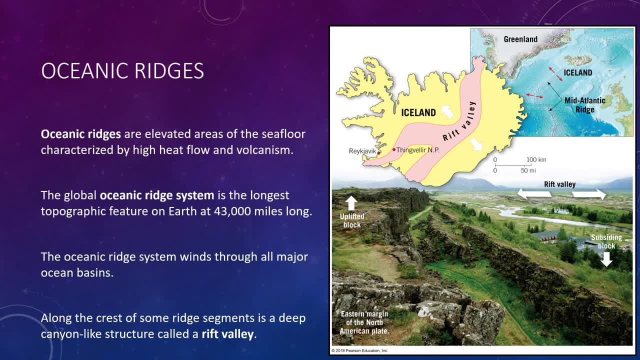 boundaries are associated with oceanic ridges. These are elevated areas of the seafloor characterized by high heat flow and volcanism. The Global Oceanic Ridge System is the longest topographical feature on Earth's surface, exceeding 43,000 miles in length. 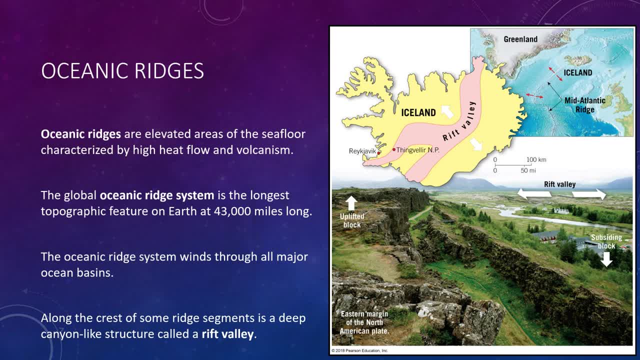 Various segments of the globe ridge system have been named, including the Mid-Atlantic Ridge, the East Pacific Rise and the Mid-Indian Ridge, Representing 20% of Earth's surface, the Oceanic Ridge System winds through all major ocean basins. 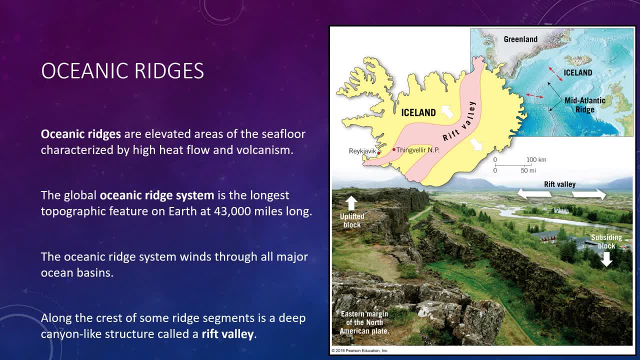 like the seams on a baseball. Although the crest of the Oceanic Ridge is commonly 2 miles higher than the adjacent ocean basin, the term ridge may be misleading because it implies narrow, when in fact it varies in width from 600 to more than 2,500. 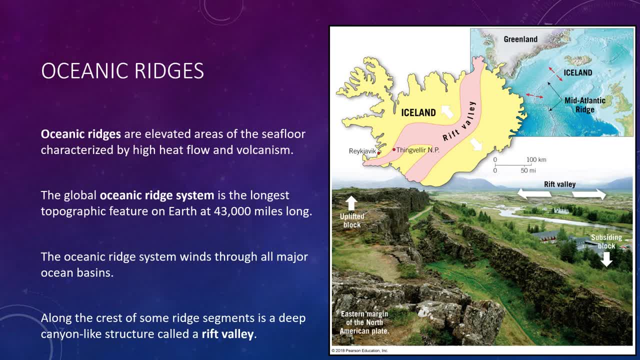 miles Further, along the crest of some ridge segments is a deep canyon-like structure called a rift valley. This structure is evidence that tensional forces, that is, pulling apart forces, are actively pulling the ocean crest apart at the ridge crest. So at this point, 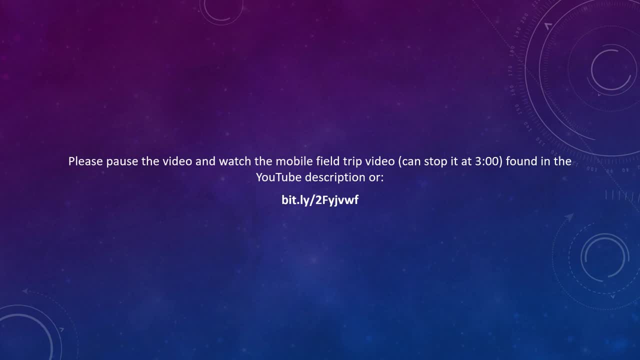 please pause the video and look at the YouTube description for a link to a mobile field trip video In notes. you can stop it after 3 minutes. The mechanism that operates along the Oceanic Ridge System to create new seafloor is appropriately called seafloor. 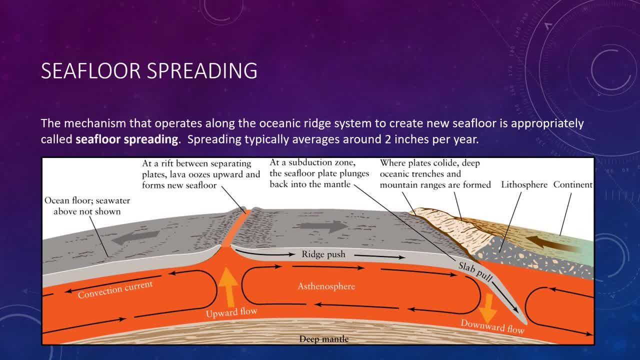 spreading Spreading typically averages around 2 inches per year, which is roughly the same rate that a human family would have to have to grow. Comparatively slow spreading rates of just over 3 quarters of an inch per year are found along the 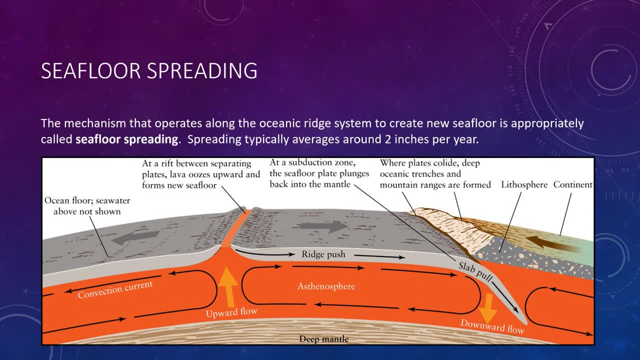 Mid-Atlantic Ridge, whereas spreading rates exceeding 6 inches per year have been measured along sections of the East Pacific Rise. Although these rates of seafloor production are slow on a human timescale, they are rapid enough to have generated all of Earth's. 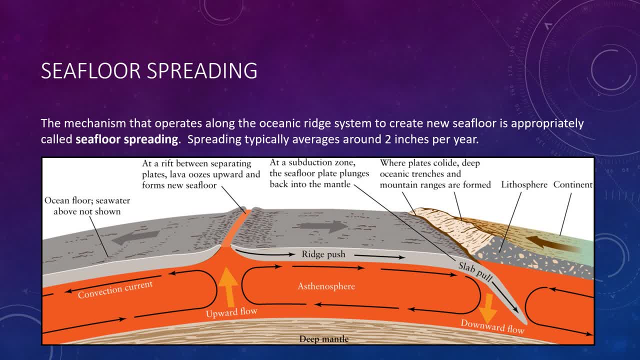 current oceanic. the primary- excuse me, the primary- reason for the elevated position of the oceanic ridge is that newly created oceanic lithosphere is hot and therefore less dense, and then the cooler rock located away from the ridge axis. as soon as the new lithosphere forms at the center, it is slowly 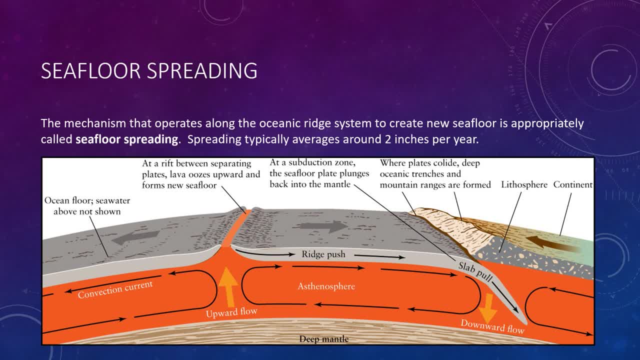 yet continuously displaced away from the zone of mantle upwelling. thus it begins to cool and contract, thereby increasing in its density. this thermal contraction accounts for the increase in ocean depth away from the ridge crest. it takes about 80 million years for the temperature of oceanic lithosphere to stabilize and contraction to cease. by this time, rock that was once part of 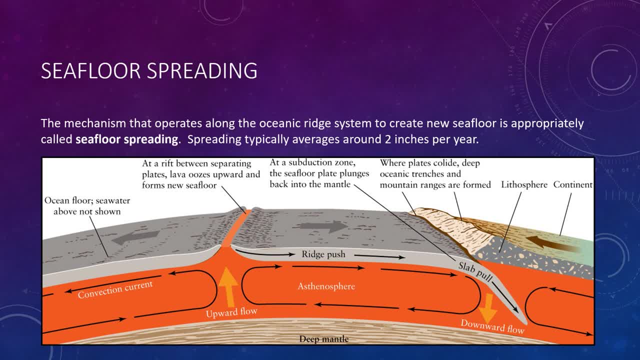 the elevated oceanic ridge system is located in the deep ocean basin, where it may be buried by substantial accumulation of the oceanic lithosphere sediment. in addition, as the plate moves away from the ridge, cooling of the underlying athenosphere causes its upper layers to become increasingly rigid and hence to become part of. 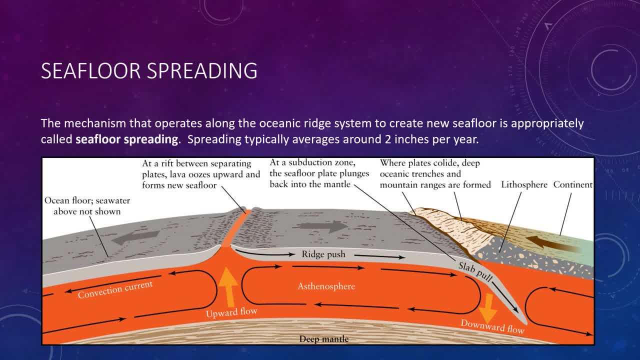 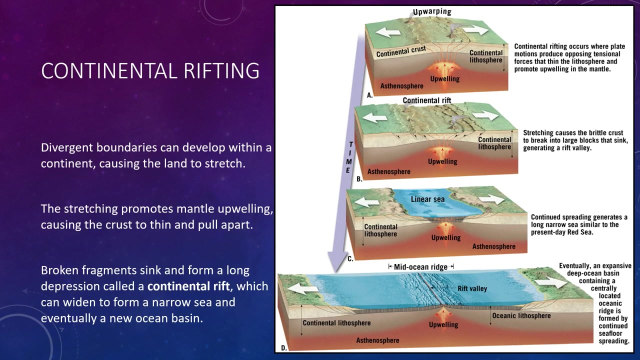 the lithosphere stated another way. the thickness of oceanic lithosphere is age dependent. lost track here. the older and cooler it is, the greater its thickness. oceanic lithosphere that exceeds 80 million years in age is about 60 miles thick approximately its maximum thickness. 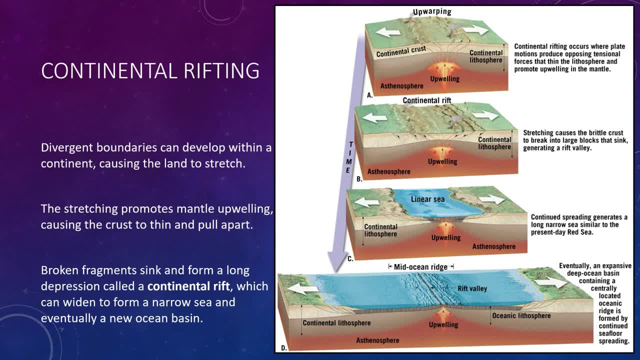 divergent boundaries can develop within a continent and may cause the land mass to split into two or more smaller segments, separated by an ocean basin. continental rifting begins where plate motions produce tensional forces that pull and stretch the lithosphere. the stretching in turn promotes mantle. 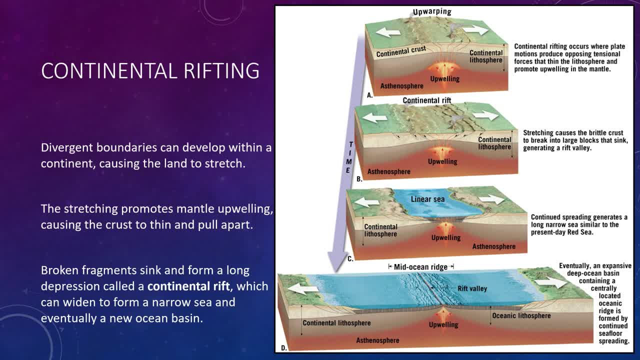 upwelling and broad upwelling to the lower platforms of the crater itself. so the stretch of the lithosphere, warping of the overlying lithosphere. This process thins the lithosphere and breaks the brittle crust rocks into larger blocks As the tectonic forces continue to pull apart the crust. 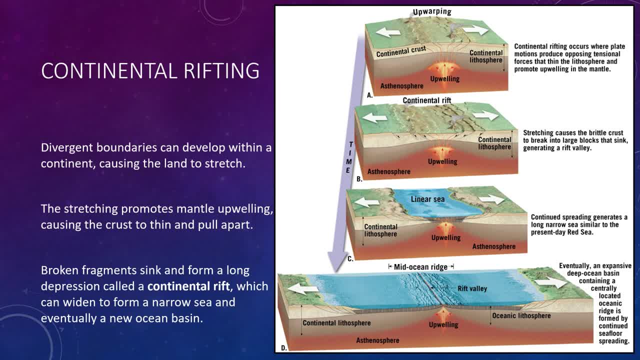 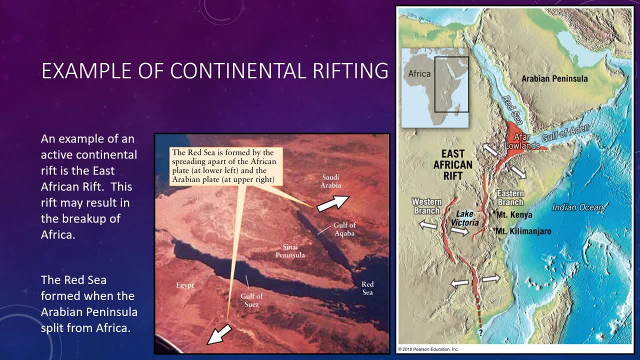 the broken crustal fragments sink, generating an elongated depression called a continental rift, which can widen to form a narrow sea and eventually a new ocean basin. An example of an active continental rift is the East African Rift. Whether this rift will eventually result in the breakup of Africa is a topic of ongoing research. Nevertheless, 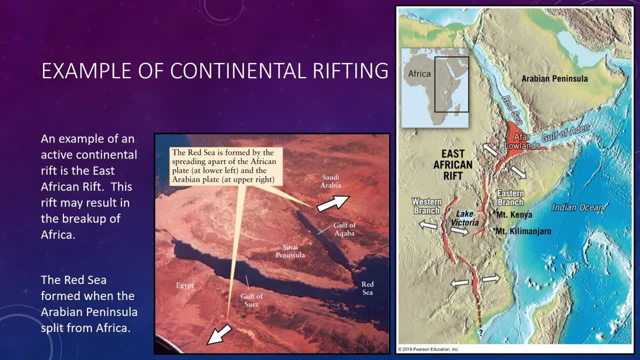 the East African Rift is an excellent model of the initial stage of the breakup of a continent. Here, tangential forces have stretched and thinned the lithosphere, allowing molten rock to ascend from the mantle. Evidence for this upwelling is that the rift has been stretched and thinned from the mantle. Evidence for this upwelling is: 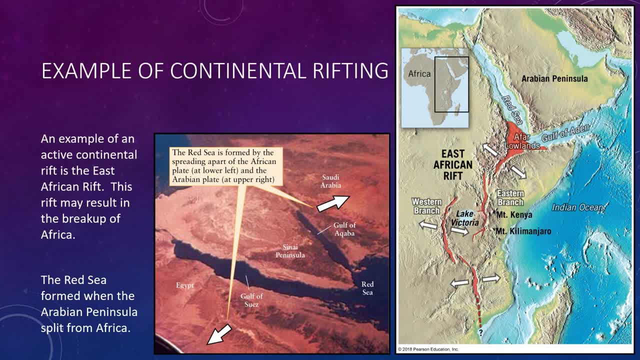 that the rift has been stretched and thinned from the mantle. Evidence for this upwelling includes several large volcanic mountains, including Mount Kilimanjaro and Mount Kenya, the tallest peaks in Africa. Research suggests that if rifting continues, the rift valley will lengthen and 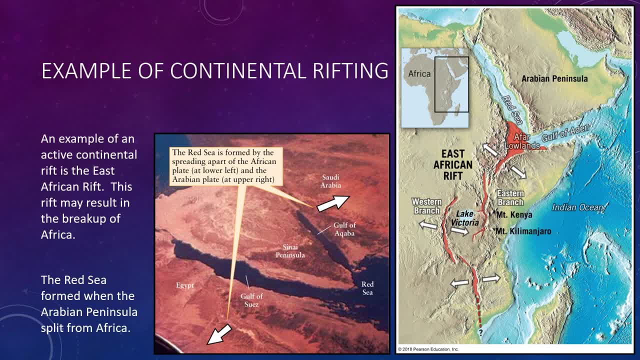 deepen at some point and the rift valley will become a narrow sea with an outlet to the ocean. The Red Sea, which is up at the top here, formed when the Arabian Peninsula split from Africa to Africa. This is a modern example of such a feature. 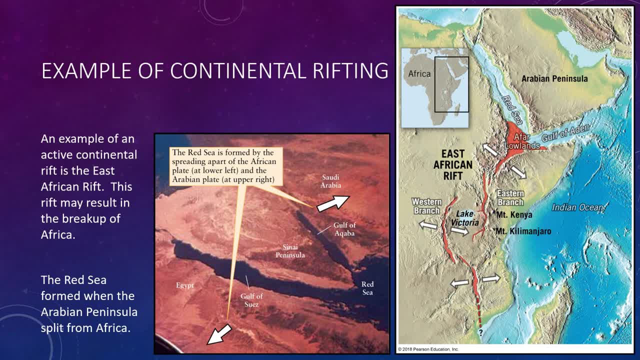 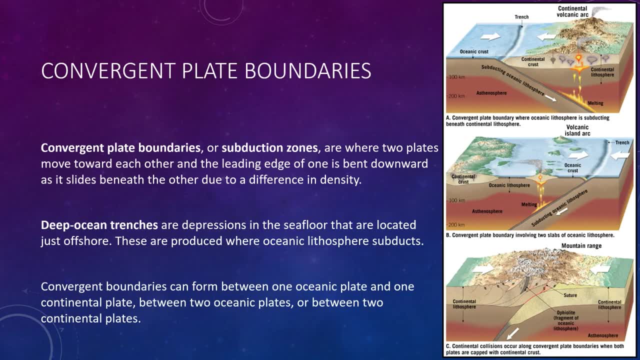 and provides us with a view of how the Atlantic Ocean may have looked in its infancy. Next we can talk about convergent plate boundaries. So there we were talking about diverging when they move apart. well, let's look at the opposite scenario, when they move together. 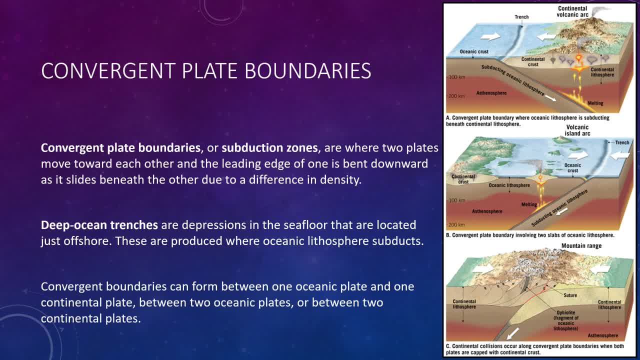 New lithosphere is constantly being produced at the oceanic ridges. However, our planet is not growing larger. Its total surface area remains constant. A balance is maintained because older, denser portions of the oceanic lithosphere descend into the mantle at a rate equal to seafloor production. 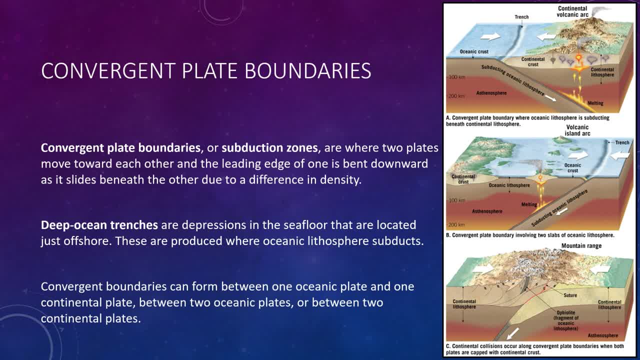 This activity occurs along convergent plate boundaries, where two plates move toward one another and the leading edge of one happens to be bent downward as it slides beneath the other. Convergent boundaries are also called subduction zones, because they are sites in which the 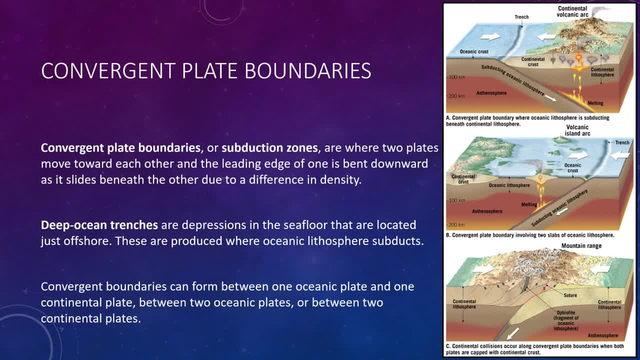 lithosphere is descending or being subducted into the oceanic ridges. Convergent plate boundaries are also called subduction zones because they are sites in which the lithosphere is descending or being subducted into the oceanic ridges. Lithospheric plates subduct because their density is greater than the density of the 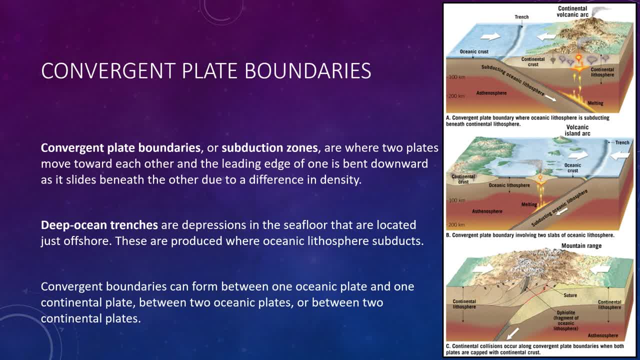 underlying athenosphere. Recall that oceanic crust has a greater density than continental crust because it is largely composed of dense, ferromagnesium rich materials. In general, old oceanic lithosphere is about 2% more dense than the underlying athenosphere. 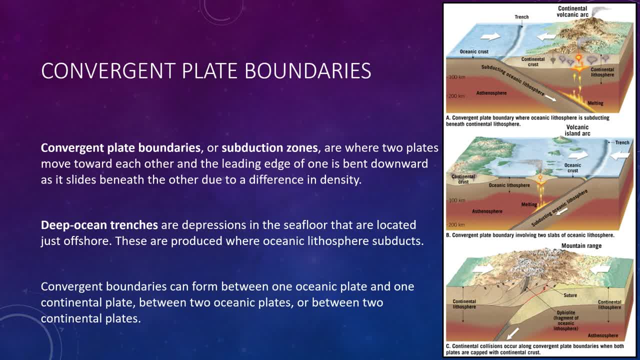 and so it sinks much like an anchor on a ship. Thus, when the exoskeleton sinks, distant particles of lithosphere sunny well. So if we put theга smiled down into the mantle and�들im the mollusc nul. Continental lithosphere, in contrast, is less dense than the underlying athenosphere and tends 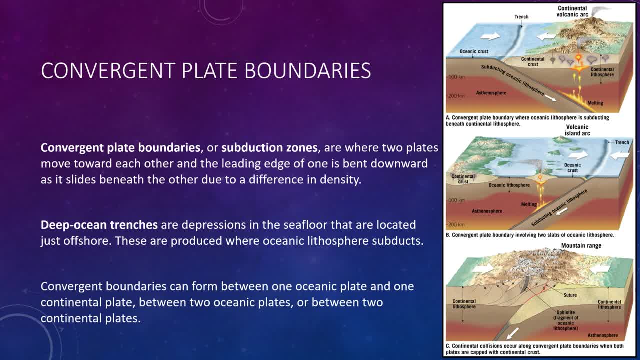 to resist subduction. However, there are, of course, a few locations where continental lithosphere is thought to have been forced below an overriding plate, albeit to relatively shallow depths. Deep ocean trenches are long linear depressions in the seafloor that are generally located only 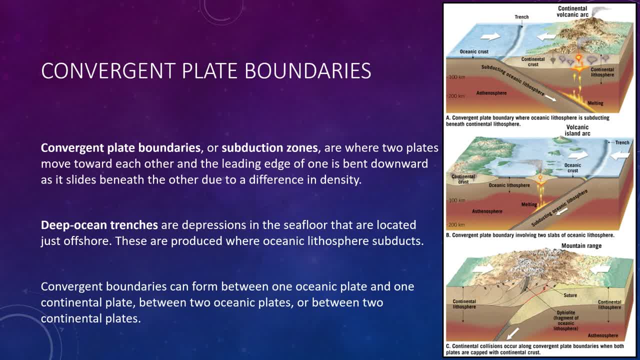 a few hundred kilometers offshore of either a continent or a chain of volcanic islands, such as the Aleutian chain off the coast of Alaska. These underwater surface features are produced where oceanic lithosphere bends as it descends into the mantle along subduction zones. 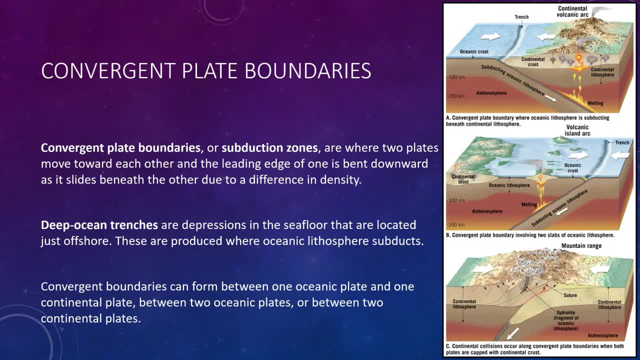 An example is the Peru-Chile Trench, located along the west coast of South America. It is more than 3,000 miles long and its floor is as much as five miles high. The trench is located on the west coast of South America. 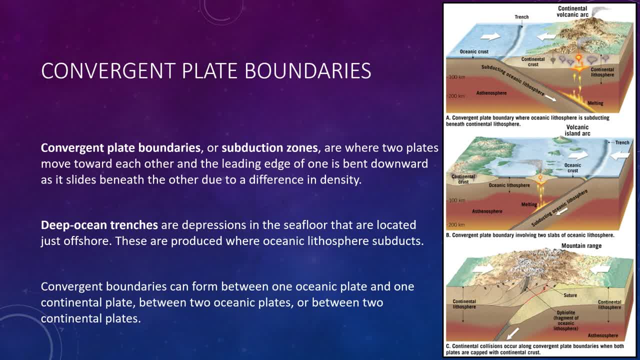 below sea level. Western Pacific trenches, including the Mariana and Tonga trenches, are even deeper than those of the eastern Pacific. Slabs of oceanic lithosphere descend into the mantle at angles that vary from just a few degrees to being nearly vertical: 90 degrees. 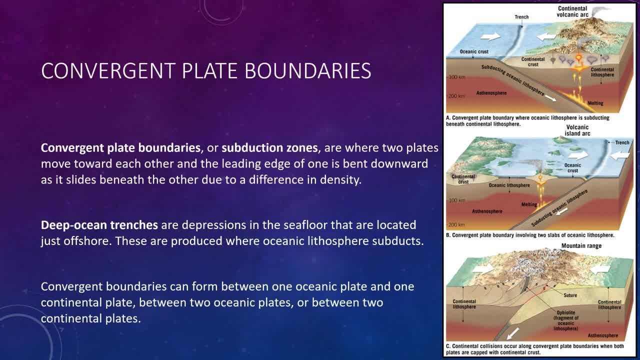 The angle at which oceanic lithosphere subducts depends largely on its age and therefore its density. For example, when seafloor spreading occurs relatively near a subduction zone, as is the case along the coast of Chile, the subducting lithosphere is 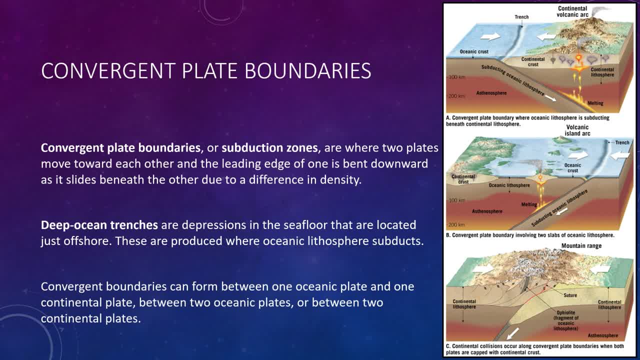 young and buoyant, which results in a low angle of descent. As the two plates converge, the overriding plate scrapes over the top of the subducting plate, a type of forced subduction. Consequently, the region around the Peru-Chile Trench experiences great earthquakes. 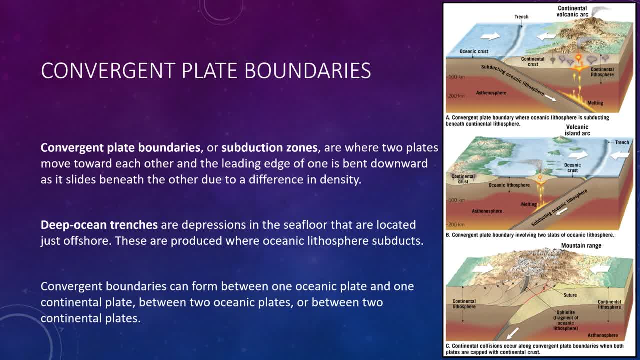 including the 2010 Chile earthquake, which was one of the ten largest on record, As oceanic lithosphere is more than a hundred kilometers long. the subducting lithosphere is larger and as the lithosphere ages, it gradually cools, which causes it to thicken and increase in. 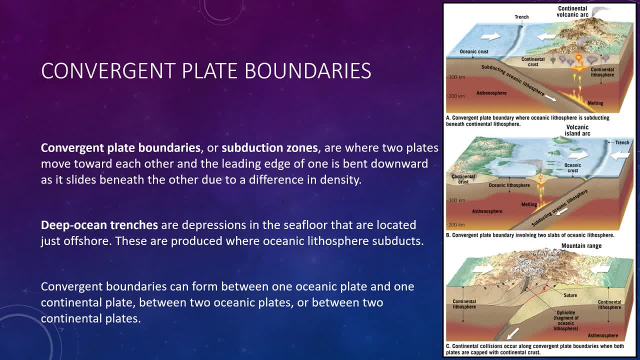 density In parts of the western Pacific. some oceanic lithosphere is 180 million years old, the thickest and densest in today's oceans. The very dense slabs in this region typically plunge into the mantle at angles approaching 90 degrees. This largely explains why most trenches 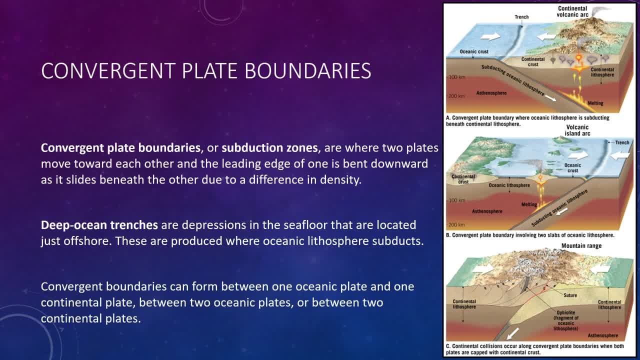 in the western Pacific are more dense than those in the western Pacific. Although all convergent zones have the same basic characteristics, they may vary considerably depending on the type of crustal material involved. Convergent boundaries can form between one oceanic plate and one continental plate, as in part A above, or between two oceanic plates. 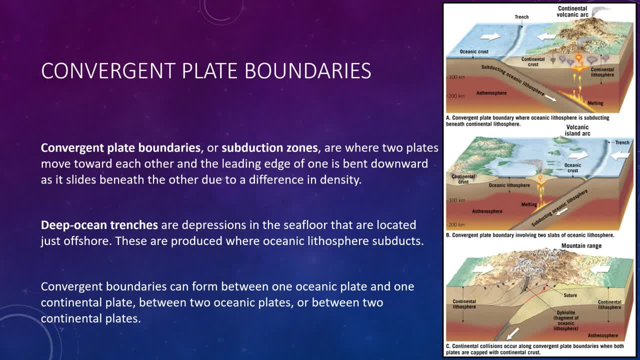 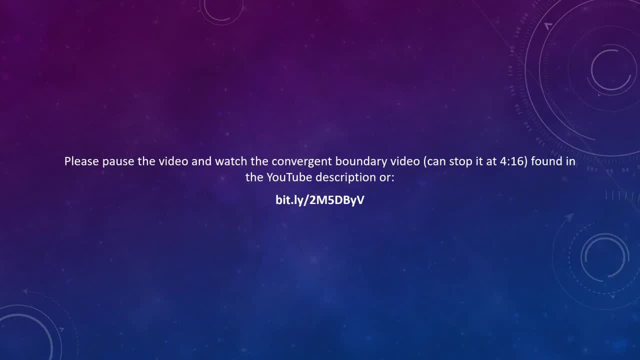 as in part B of the figure, or even between two continental plates, as in part C. So at this moment, please pause the video and refer to the YouTube description for a convergent plate boundary video which you can stop after about 4 minutes and 16 seconds. 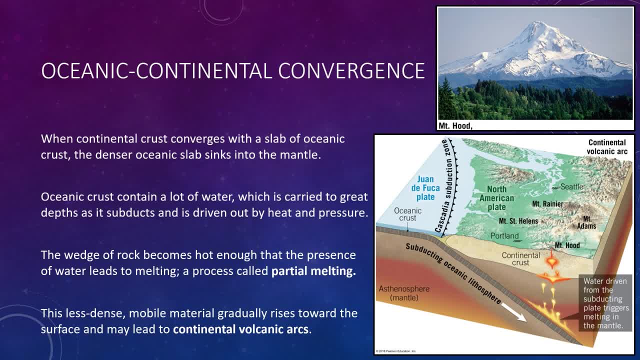 So let's go ahead and step through each of these different types. We'll start with oceanic continental convergence. When the leading edge of a plate capped with continental crust converges with a slab of oceanic lithosphere, the buoyant continental block remains. 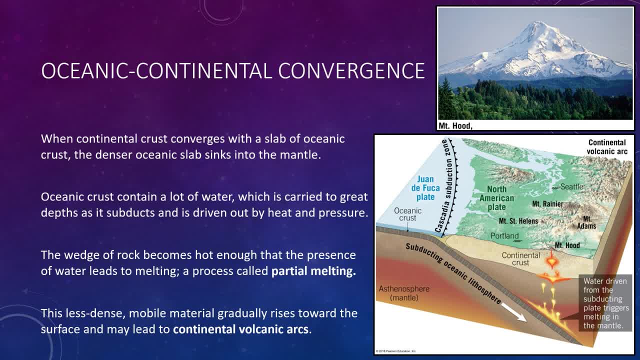 floating While the denser oceanic slab sinks into the mantle. When a descending oceanic slab reaches a depth of about 60 miles, melting is triggered within the wedge of hot athenosphere that lies slightly above it. But how does the subduction of a cool slab of oceanic lithosphere cause melting of mantle rock? 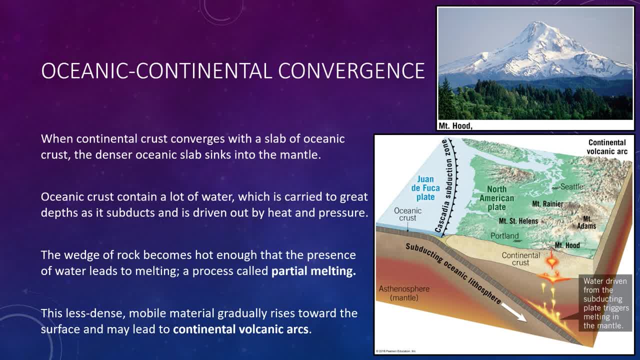 Well, the answer lies in the fact that water contained in the descending plates acts the way salt does to melt ice, That is, wet rock melts into the mantle. So the rock in a high pressure environment melts at a substantially lower temperature than dry rock does. 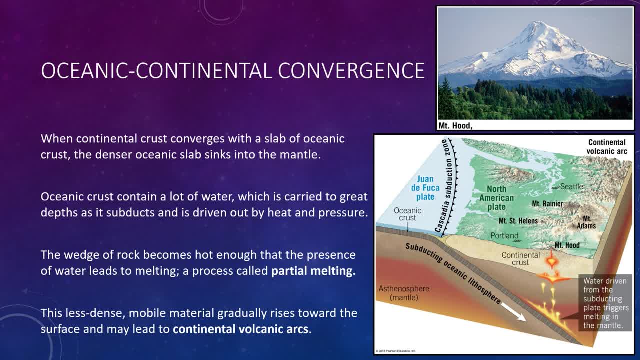 Sediments and oceanic crust contain large amounts of water which is carried to great depths by the subducting plate. A lot of water on this piece it carries down below As the plate plunges downward, heat and pressure drive the water out from the hydrated minerals in the subducting slab. 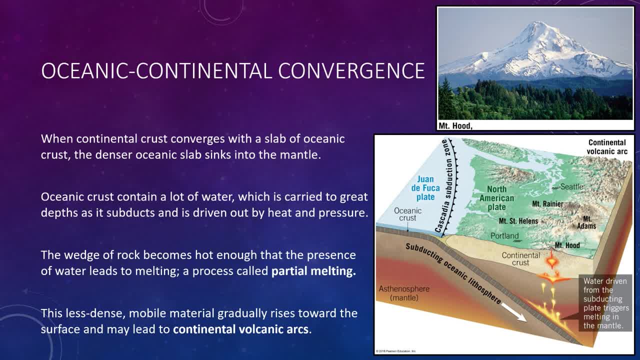 At a depth of about 60 miles. the water is lost in the subduction slab At a depth of about 60 miles. the water is lost in the subducting slab At a depth of about 60 miles. the water is lost in the subducting slab. 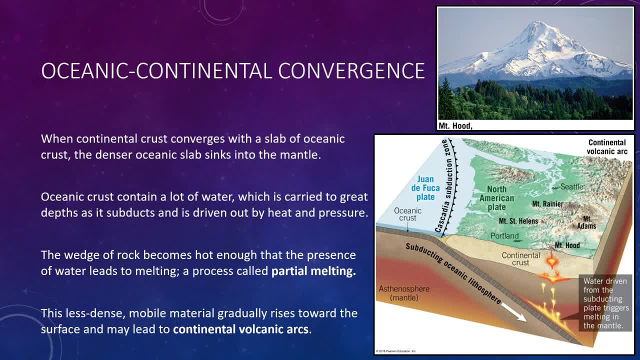 60 miles. the wedge of mantle rock is sufficiently hot enough that the introduction of water from the slab below will lead to some melting. This process, called partial melting, is thought to generate molten material, which is mixed with unmelted mantle rock. 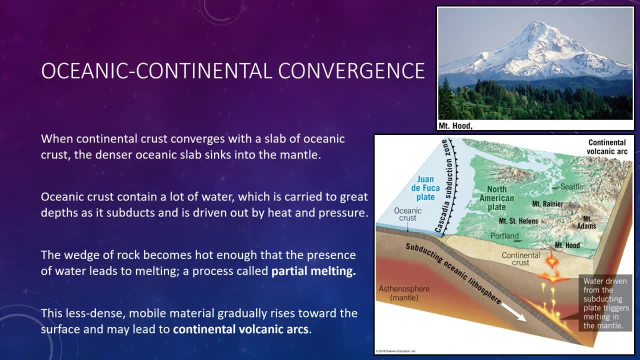 Being less dense than the surrounding mantle, this hot mobile material gradually rises toward the surface. Depending on the environment, these mantle-derived masses of molten rock may ascend through the crust and give rise to volcanic eruption. However, much of this material never reaches the surface and solidifies at depth a process. 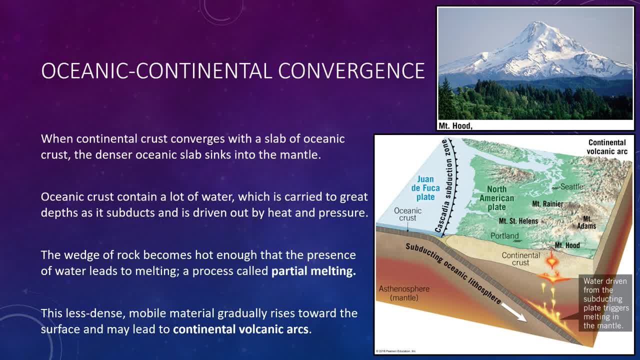 that will thicken the crust. The volcanoes of the towering Andes Mountains were produced by molten rock generated by the subduction of the Nazca Plate beneath the South American Plate Mountain systems like the Andes, which are the largest mountain systems in the world. 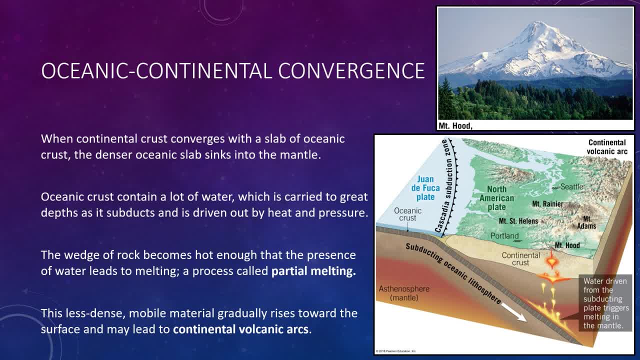 are also known as the Andes Mountains. Volcanoes which are produced in part by volcanic activity associated with the subduction of oceanic lithosphere are called continental volcanic arcs. The Cascade Range in Washington, Oregon and California is another mountain system consisting. 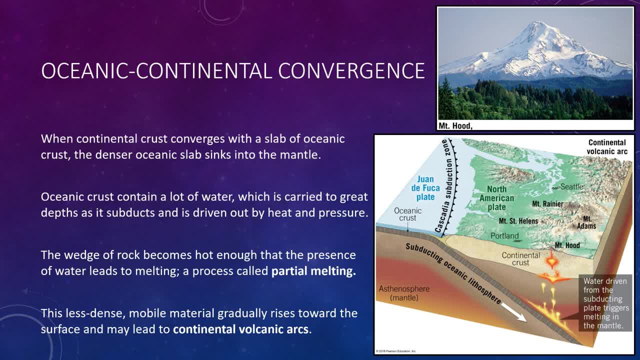 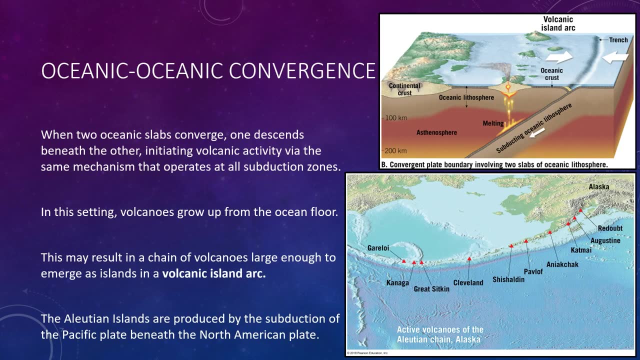 of several well-known volcanoes, including Mount Rainier, Mount St Helens and Mount Hood. This active volcanic arc also extends into Canada, where it includes Mount Jerebaldi and Mount Meagher. However, eligio and magma involvement is atg consume some of theował oceanic. 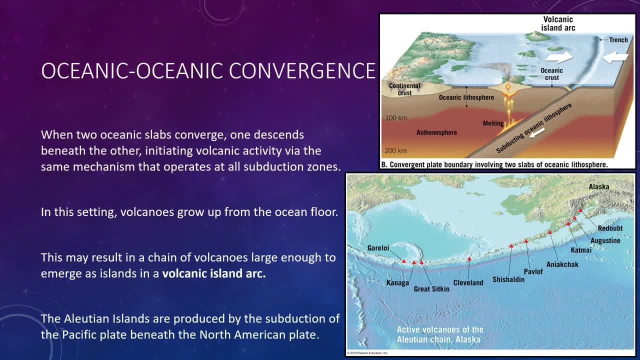 networks, The Ma'noak shopsresser. They used UN Turline and also surveillance in general. Since 760 BE講 conquered height of over 1,000 miles per hour. The Indian martymph流 was sold online at 1910.. 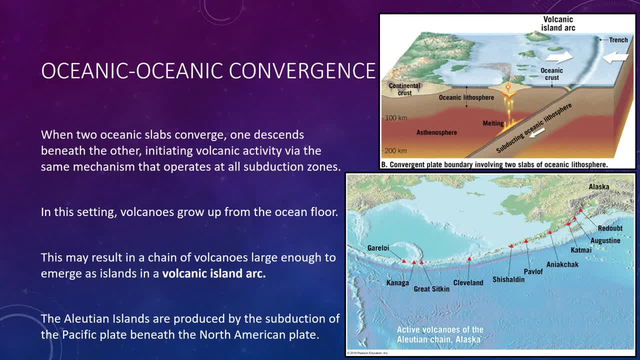 young volcanic island arcs. Island arcs are generally located 75 to 225 miles from a deep ocean trench. Located adjacent to the island arc just mentioned in the Aleutian Trench are the Aleutian Trench, the Mariana Trench and the Tonga Trench. 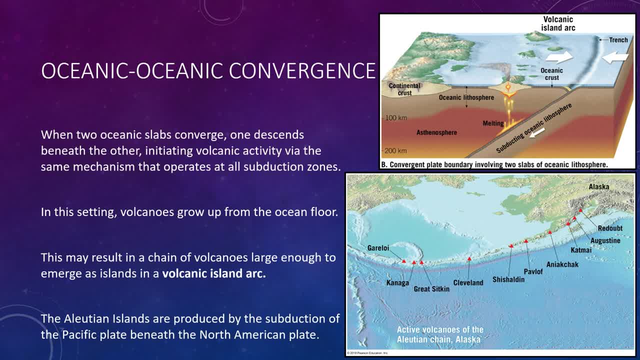 Most volcanic island arcs are located in the western Pacific. Only two are located in the Atlantic: the Lesser Antilles Arc, which is on the eastern margins of the Caribbean Sea, and the Sandwich Islands, located off the tip of South America. The Lesser Antilles are a product. 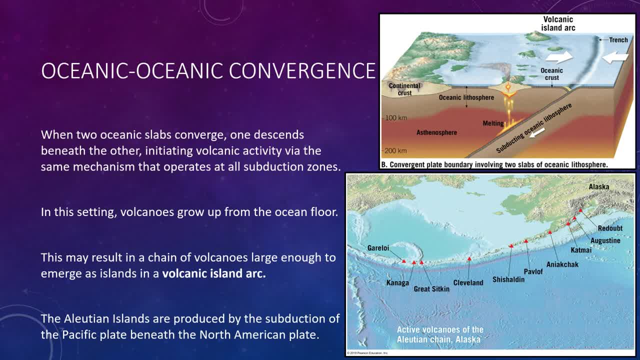 of the subduction of the Atlantic seafloor beneath the Caribbean Plate. Located within this volcanic arc are the Virgin Islands of the United States and the British Isles, as well as Mount Pele, which erupted in 1902, which destroyed the town of Saint-Pierre and killed an estimated 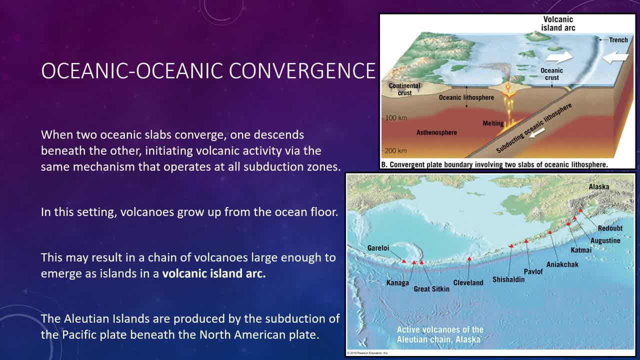 20,000 people. The Lesser Antilles Arc is located on the eastern margins of the Caribbean Sea- 28,000 people. This chain of islands also includes volcanic activity that occurred as recently as 2010.. Island arcs are typically simple structures made of numerous volcanic cones underlain by 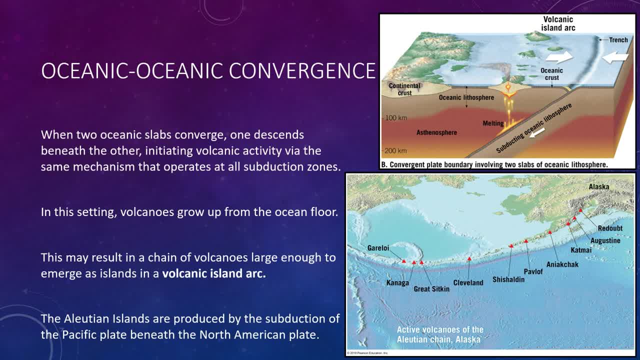 oceanic crust that is generally less than 12 miles thick. Some island arcs, however, are more complex and underlain by highly deformed crust that may reach 22 miles in thickness. Examples include Japan, Indonesia and the Alaskan Peninsula. These island arcs are built on material generated by 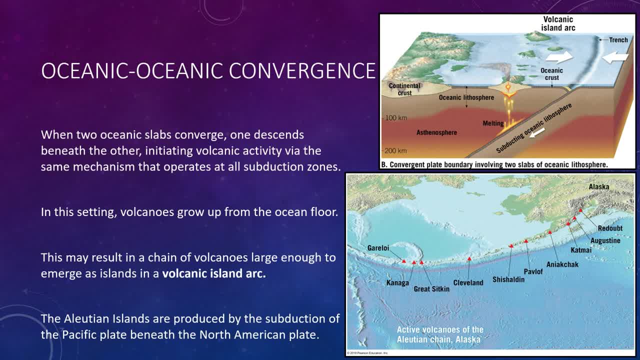 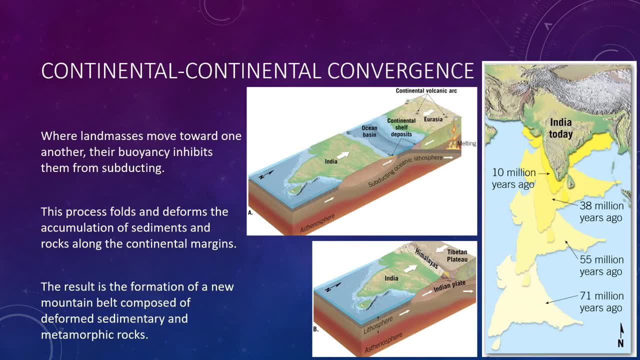 earlier episodes of subduction or on small slivers of continental crust that has rafted away from the mainland. The third type of converging plate boundaries is continental-continental convergence. In this case we have one landmass moving toward another because of subduction of 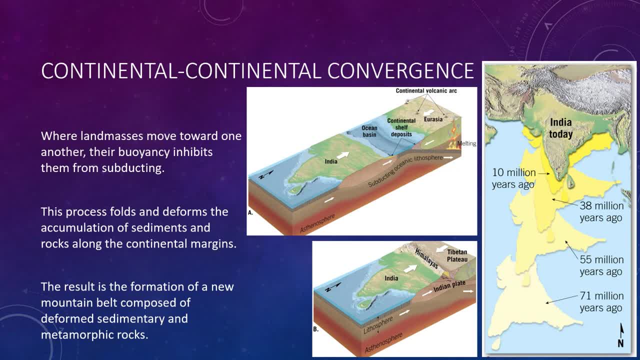 intervening seafloor. Whereas oceanic lithosphere tends to be dense and readily sinks into the mantle, the buoyancy of continental material generally inhibits it from being subducted, at least to any great depth. Consequently, a collision between two converging continental fragments ensues. 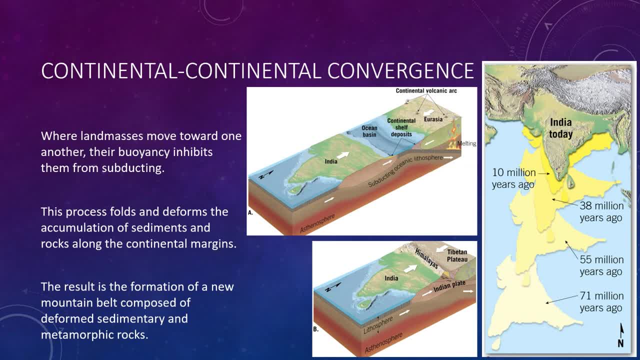 This process folds and deforms the accumulation of sediment and sedimentary rock along the continental margins, as if they had been placed in a gigantic vice. The result is the formation of a new mountain belt composed of deformed sedimentary and metamorphic rocks that contains 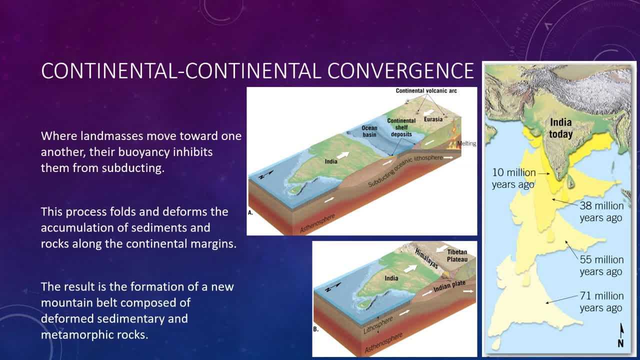 slivers of oceanic lithosphere. Such a collision began about 50 million years ago, when the subcontinent of India rammed into Asia, producing the Himalayan Mountains, the most spectacular mountain range on Earth. During this collision, the continental crust buckled and fractured. 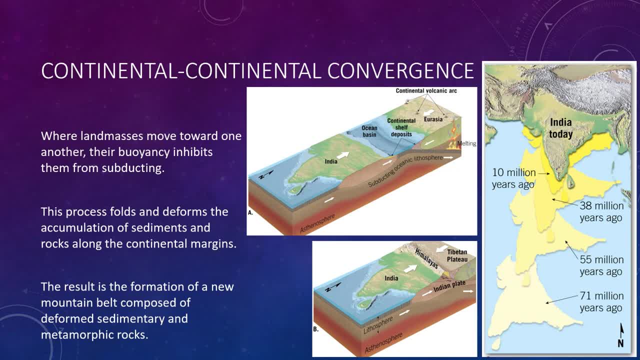 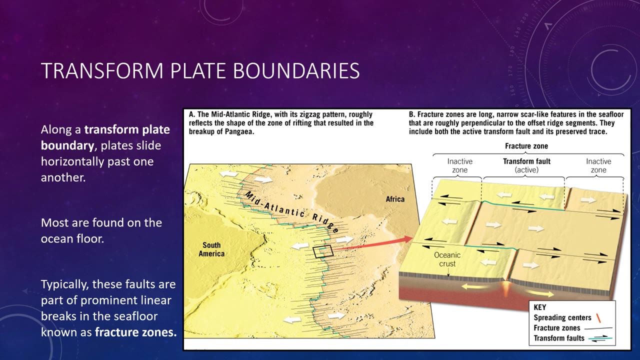 and was generally shortened horizontally and thickened vertically. In addition to the Himalayas, several other major mountain systems, including the Alps, Appalachians and the Urals, formed from continental fragments colliding. The last type of boundary that we'll look at is a transform plate: boundary Along a transform plate. 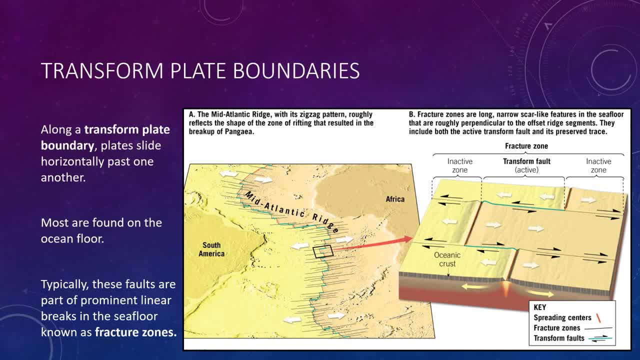 boundary, also called a transform fault. plates slide horizontally past one another without the production or destruction of the lithosphere. The nature of transform faults was discovered in 1965 by Canadian geologist J Tuzo Wilson, who proposed that these large faults connect. 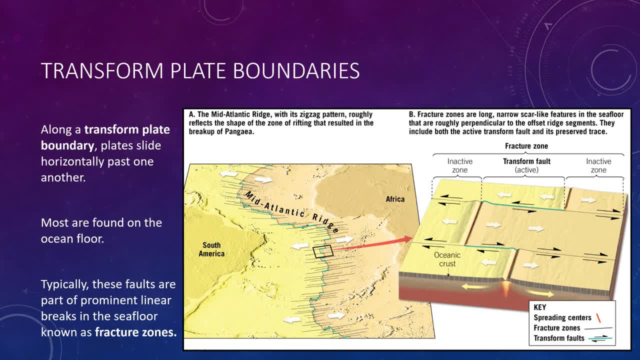 two spreading centers, divergent boundaries or, less commonly, two trenches or convergent boundaries. Most transform faults are found on the ocean floor, where they offset segments of the ocean ridge system, producing a step-like plate margin that you can see in the figure. 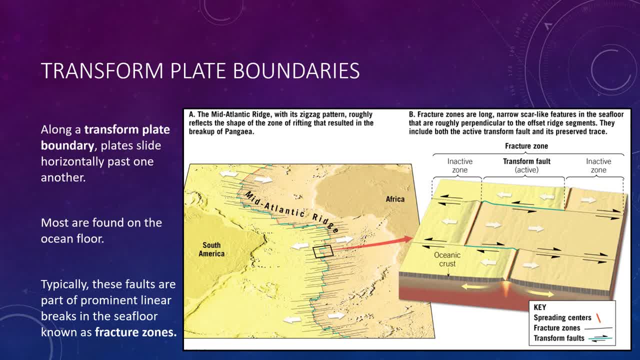 Notice that the zigzag shape of the mid-Atlantic Ridge is. the shape of the mid-Atlantic Ridge roughly reflects the shape of the original rifting that caused the breakup of the supercontinent Pangea. Typically, transform faults are part of prominent linear breaks in the seafloor, known as 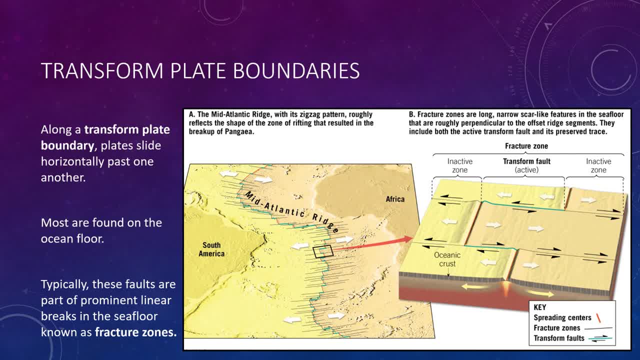 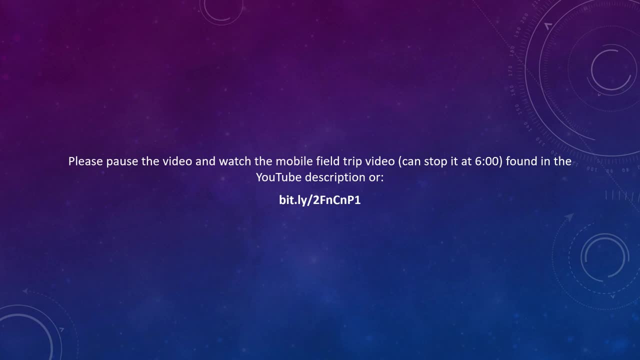 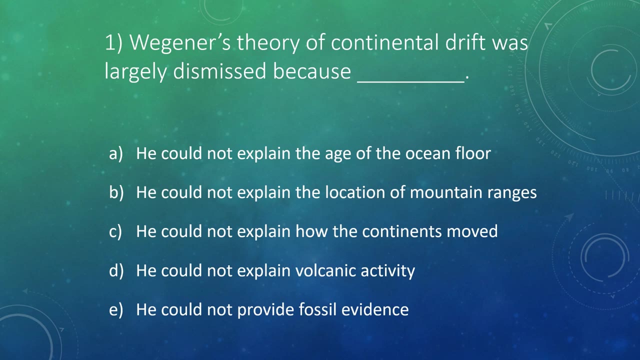 fracture zones, which include both active transform faults and their inactive extensions into the plate interior. Alright, at this point you can pause the video and watch another mobile field trip video, which you can stop after six minutes From here. let's go ahead and close out this first lecture on plate tectonics with a few questions. 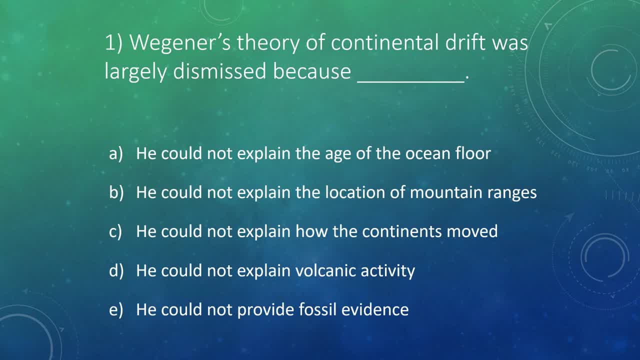 So, as always in this case, I'll read the question. then you should pause the video while you contemplate the answer and then resume it when you have an answer ready. So question number one, Wagner's theory of continental drift, was largely dismissed because 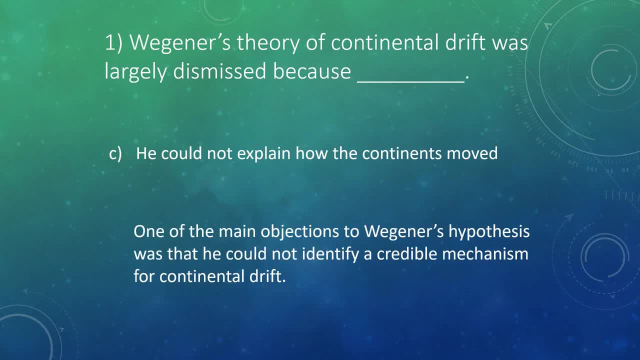 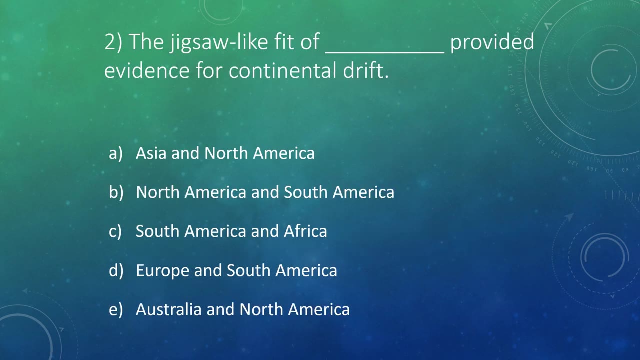 what? The answer here is: C: He could not explain how the continents moved. Remember, he came up with the idea of the tides of the sun and moon affecting continental motions, which, of course, is not true today. Number two: The jigsaw-like fit of blank provided. 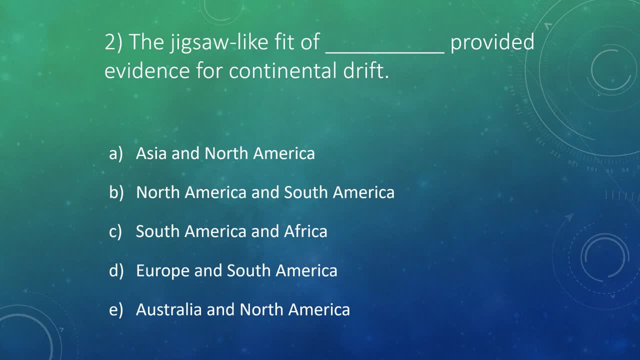 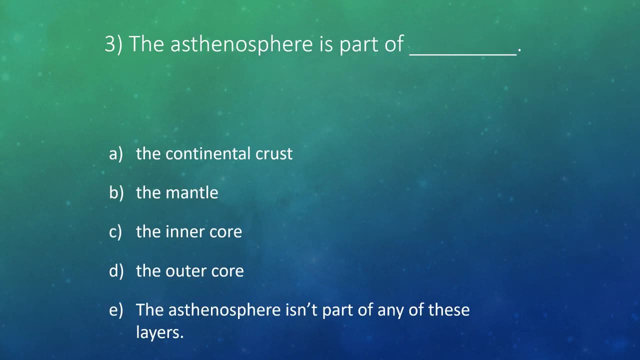 evidence for continental drift. Well, we saw the fit of South America and Africa. Answer C: We have a wonderful fit between their oceanic boundaries. Number three: The asthenosphere is part of what The asthenosphere is part of B the mantle, It's a hotter. 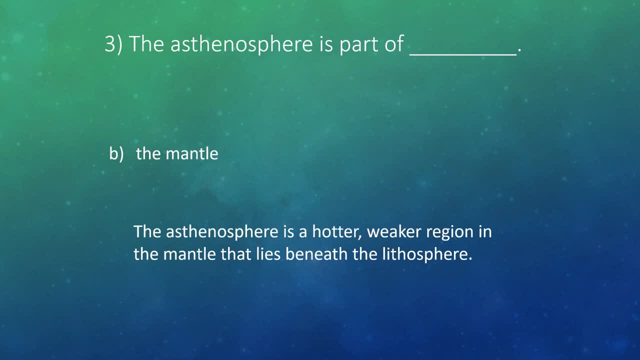 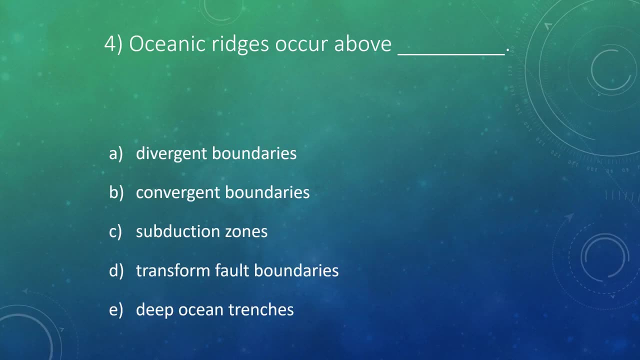 weaker region in the mantle that lies beneath the harder outside region of the lithosphere? Question four: Oceanic ridges occur above what? In this case we see them occur above diatoms. So oceanic ridges form at all divergent boundaries, So when two plates are moving apart,